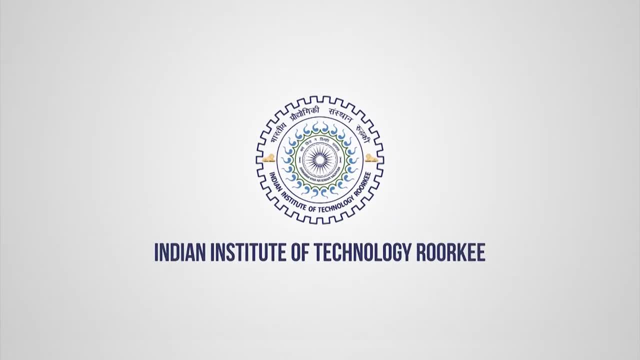 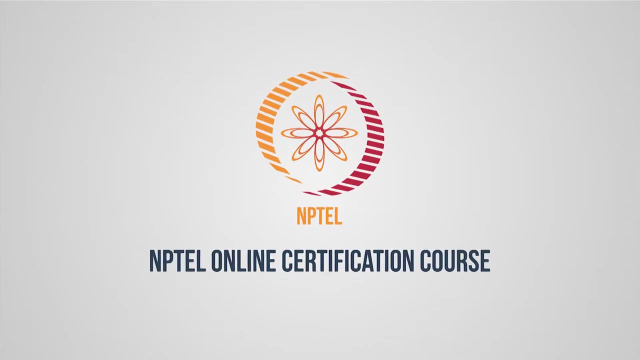 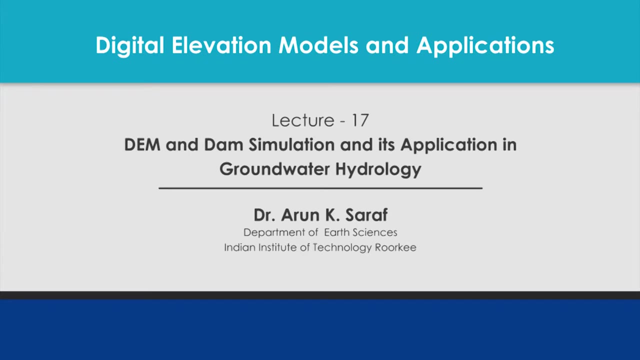 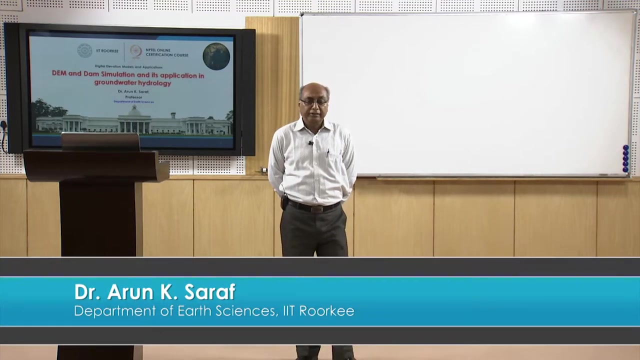 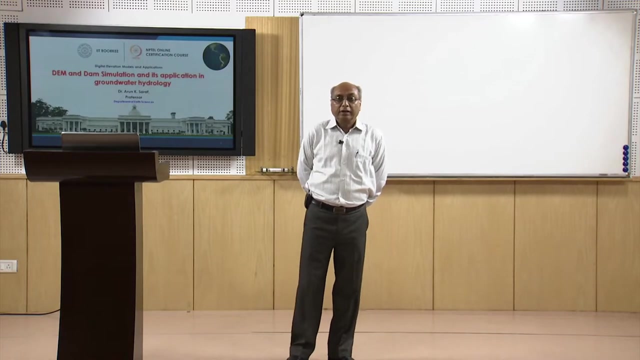 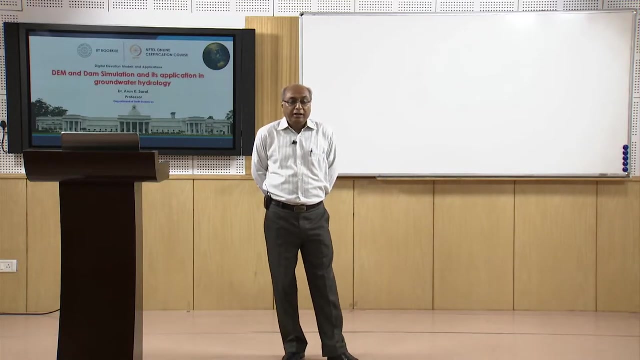 Hello everyone and welcome to digital elevation models and application course. This is the 17th lecture of this course and in this one we are going to discuss how digital elevation model can be used for dam simulations, that is, reservoir simulations, DAM- and how this simulation can help us in groundwater related studies. So this is another way of using. 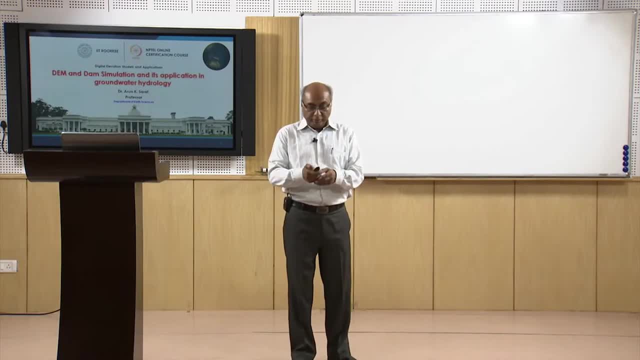 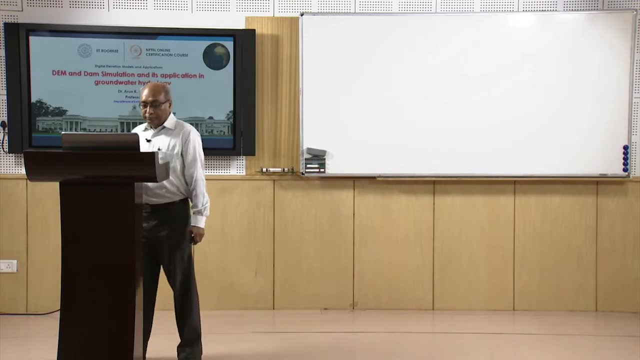 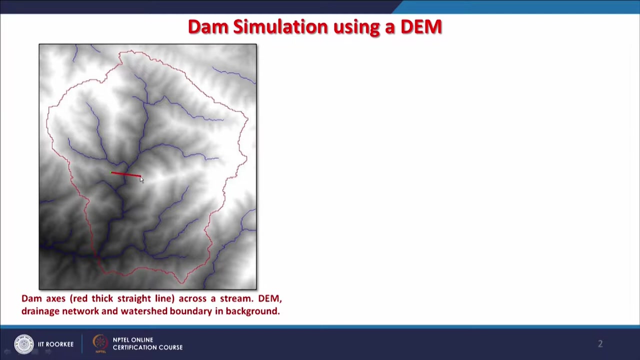 digital elevation model, or one can call as a derivative of digital elevation model. Again, we are going to take the same example of digital elevation model here, and what I am showing here is there is a dam axis which has been drawn over the digital elevation model, As you can see very clearly that there is a red line. So this is the dam axis, and 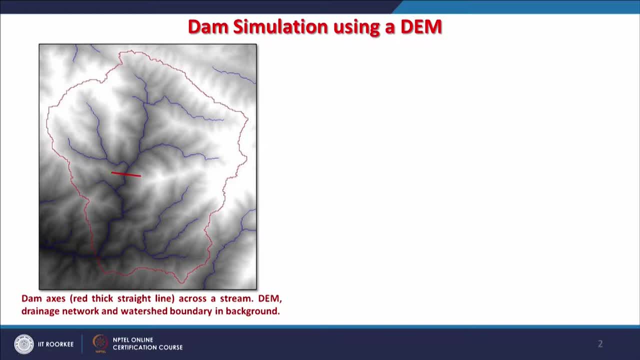 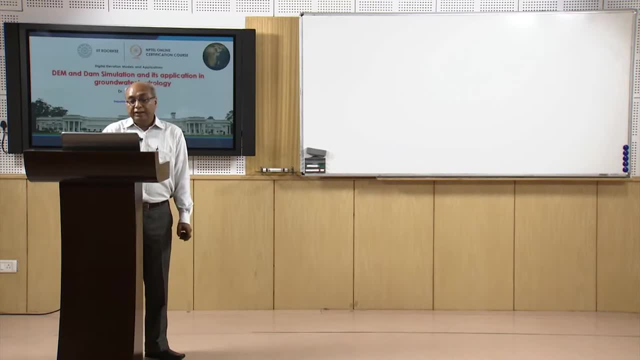 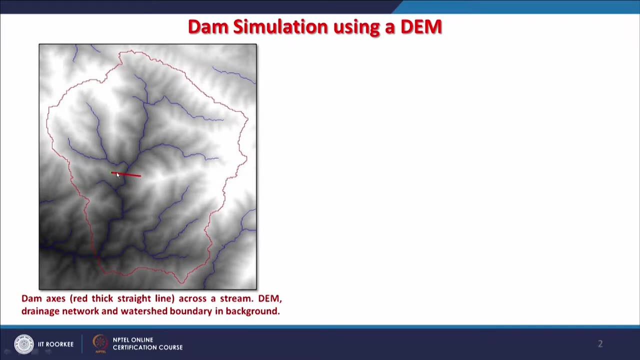 across a stream. This has been drawn Now in dam simulations, the facilities which are available. anytime I can change the length of this line. I can change the direction of this line and roughly at present it is east-west. I can change to other directions But as you will see that, 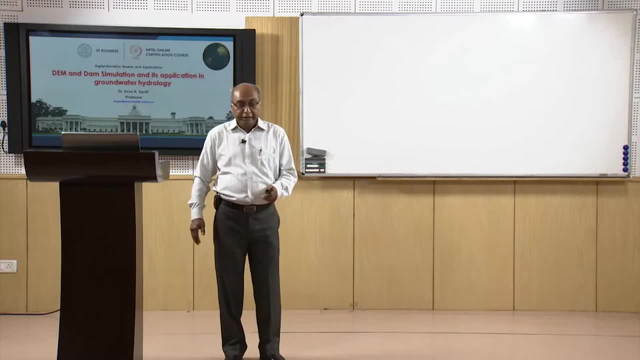 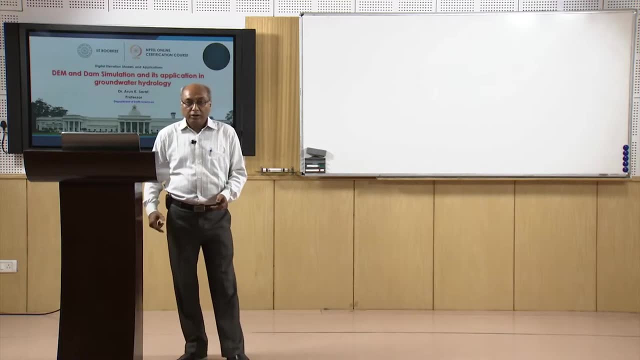 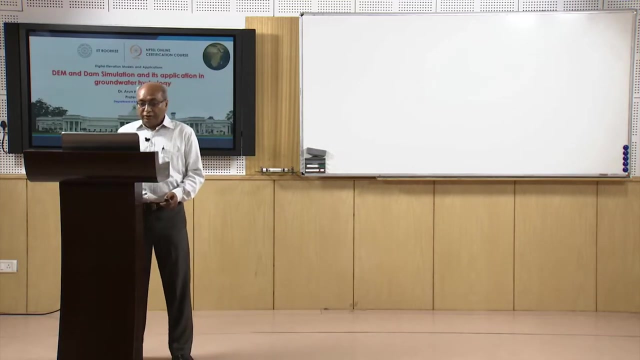 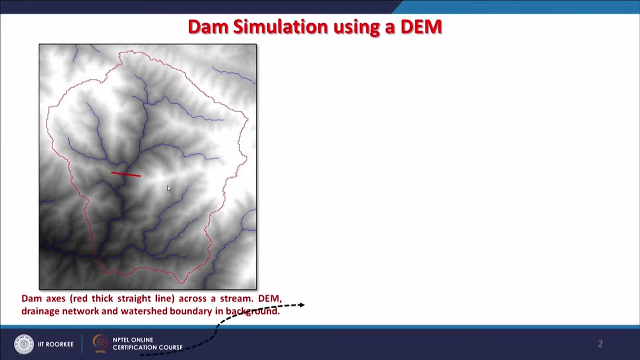 it is not really required to change too much because, after all, what we are going to? use this digital elevation model for dam simulations, So it has to fill the water and therefore we will keep in this particular example, this dam axis like this and this, once you draw. 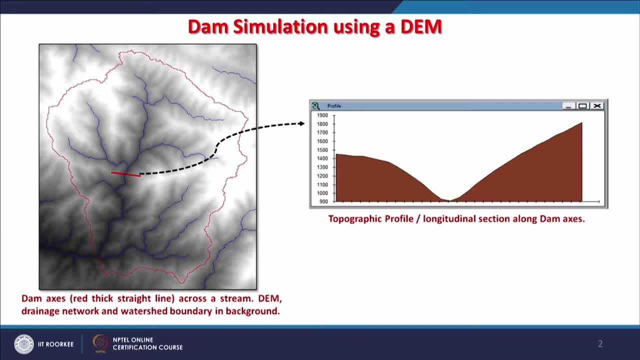 a line over a digital elevation model. the next output you can generate is the profile or topographic profile, which we have already discussed here, And this is the topography along this straight line as a dam axis. Now we are based on this. we can think that if I keep the water level as 1400 meter here, in this particular example, 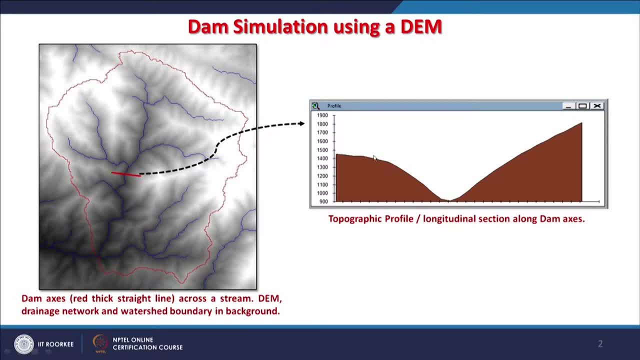 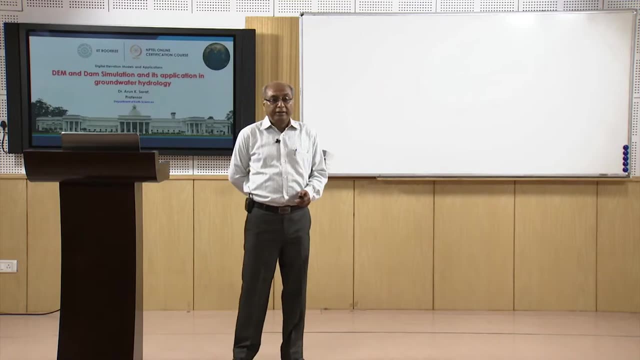 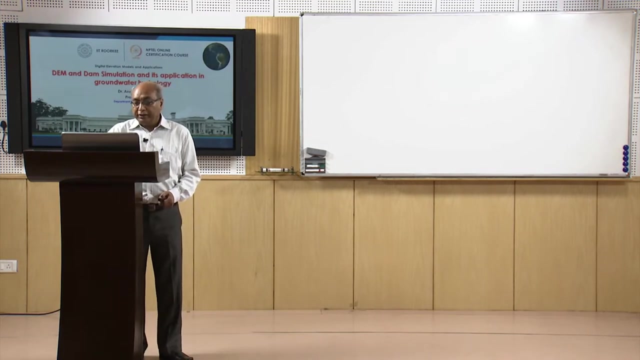 then still water will remain in between these two mounds or any high areas and I can fill or simulate the reservoir here, reservoir here. So based on the topographic profile, I can decide the height of the dam here. So here the height of the dam was kept at 1400 meter, as you can see. So in the profile. 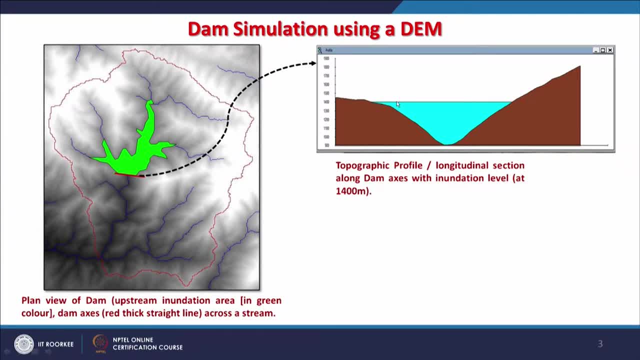 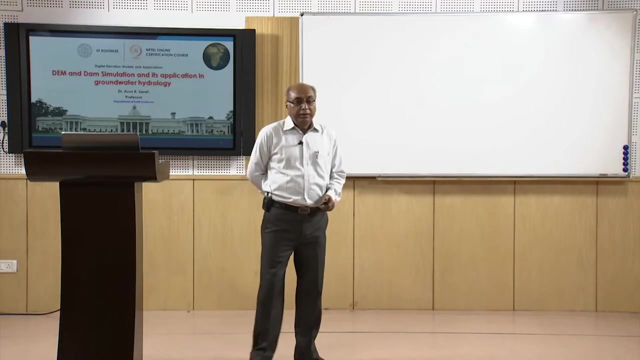 this is the section view and we are seeing that water has filled and this dam this is being used here and this is the plan view of upstream area which will be inundated if water is filled up to 1400 meter over at this dam axis And this is how very quickly a dam. 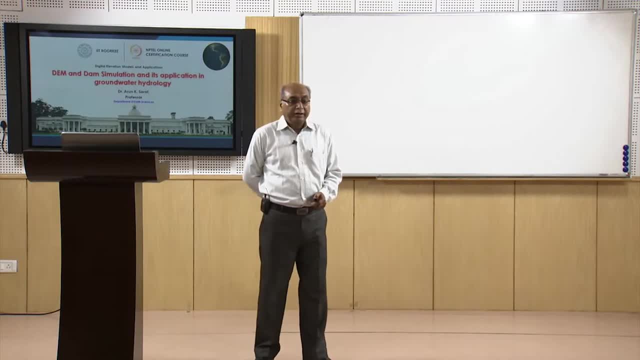 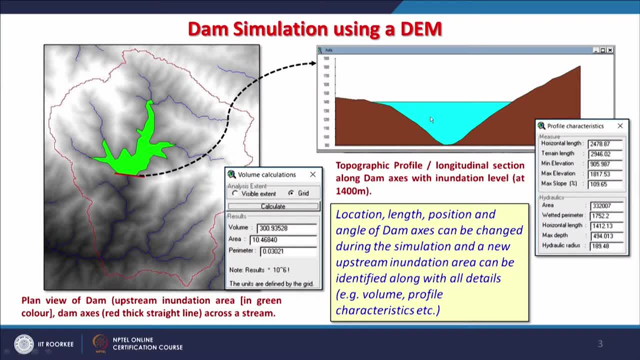 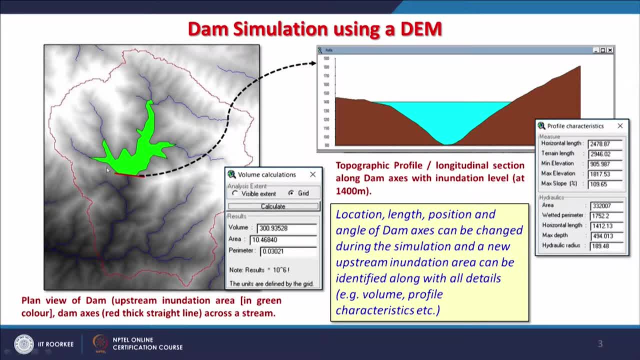 that is the length here and the total length of this stem axis, then terrain length, which is going to be more than the horizontal length. This is the terrain length, then minimum elevation. what is the minimum elevation? So this is coming around 905 here, as you can see very easily. 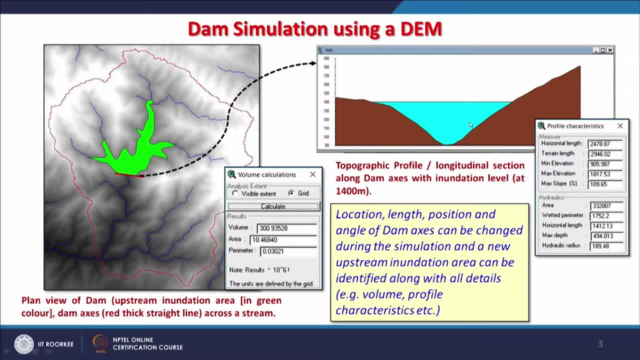 Then maximum elevation available here along this topographic profile is 1817, and then maximum slope also there. and then what other hydraulic characteristics of this topographic profile can also be calculated, like area, wetted perimeter, horizontal length, maximum depth and hydraulic radius? 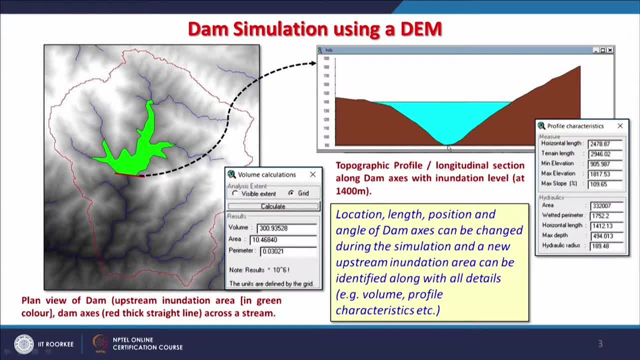 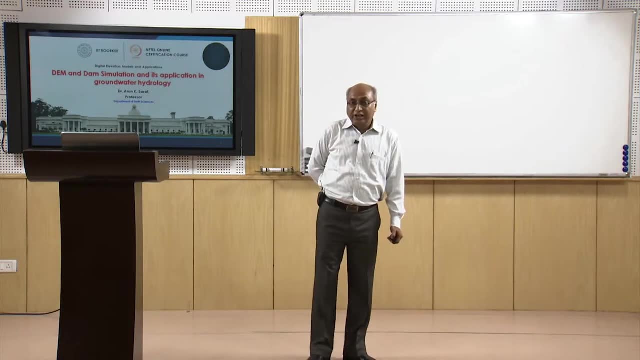 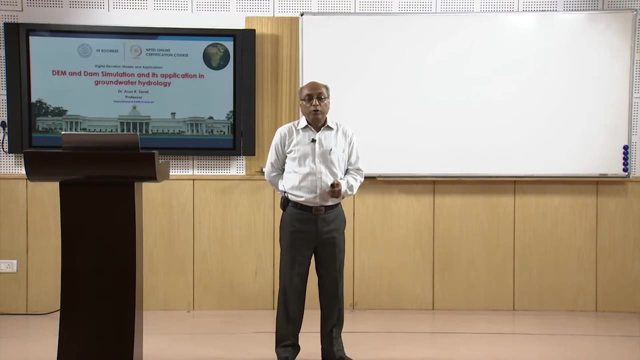 The maximum depth will be calculated somewhere here, And this is 400, sorry 494- and the maximum depth which we are getting here. So likewise, lot of parameters which are required in the designing of a dam or a reservoir can be simulated, can be estimated before anything is really constructed on a digital on it in. 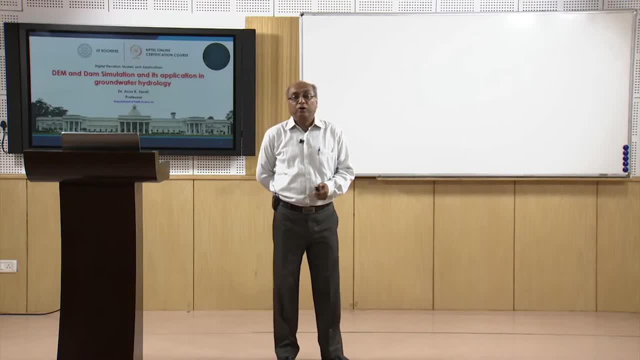 a terrain, And thus that is the biggest advantage of digital terrain: Digital elevation models- and this can be done on a GIS platform. If I give you further information about the software, then the current ArcGIS software do not have a direct tool available, but nonetheless this through several steps, this dam simulation. 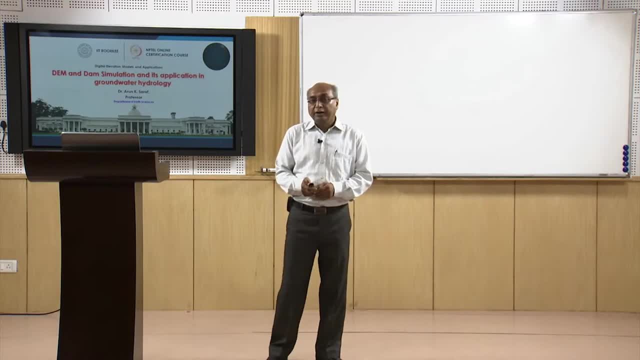 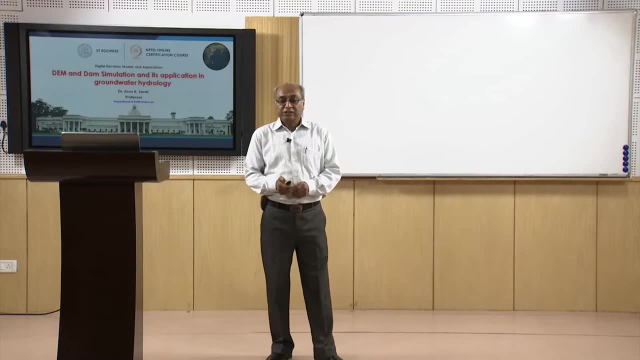 exercise can be done or this modeling can be done, Whereas in the older version, That is, ArcView 3.2, there is an extension which is called profile extractor, and using that extension this can be done very quickly in the simulation which I have shown here. 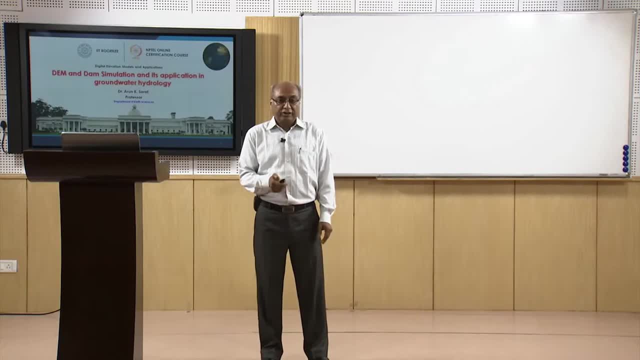 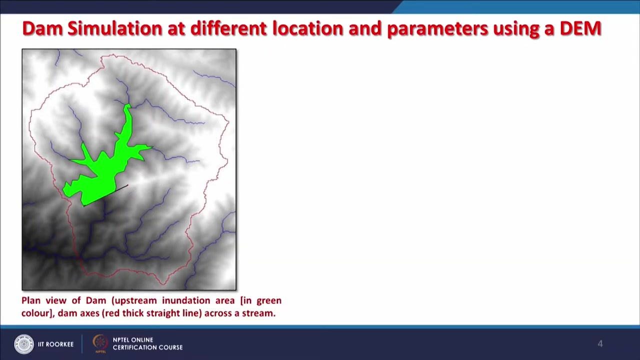 in this example is been done using profile extractor. So on ArcView GIS software. but on ArcGIS the straightforward approach or the special extension or tool is not available. But if one use through cut and fill analysis, almost the same results can be achieved. Now different locations as I have chosen. now I have changed the location in the previous. 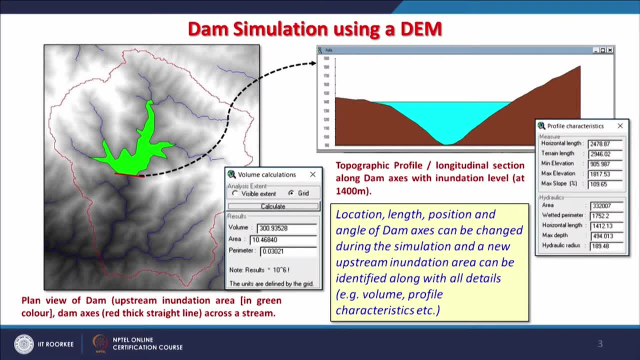 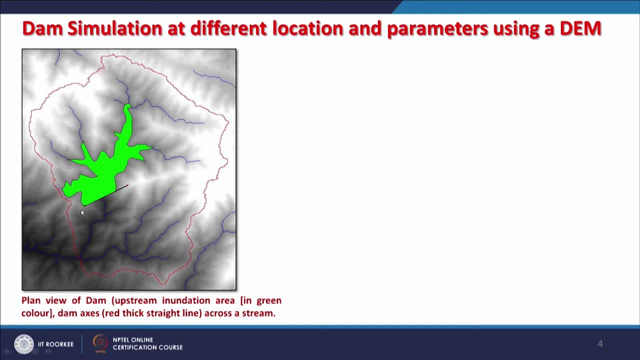 example, the dam was somewhere else. Now I have shifted the dam axis, I have changed the dam length and the result this dam axis length. So that is the advantage of simulation. so doing these exercises on a GIS platform using a digital elevation model, that one, if one is targeting a particular volume of water. 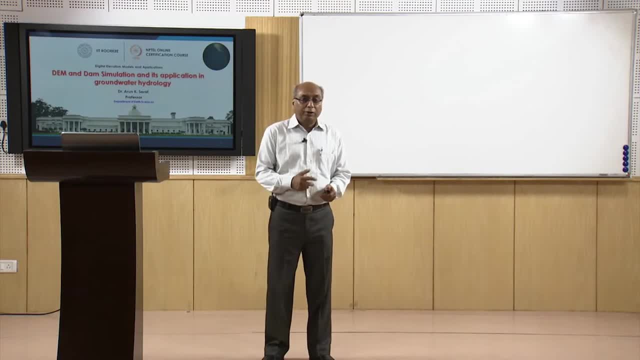 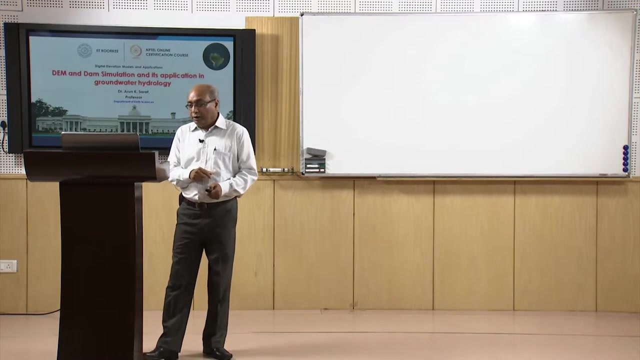 in a terrain for storage, may be for hydro power or other things- then before anything is done on the ground, all these simulations can be done and a proper decision can be reached. So that is the advantage of simulation And this derivative of a digital elevation model. of course one has to imply the GIS here. 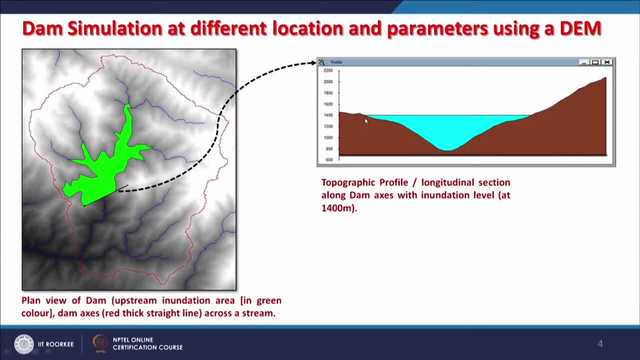 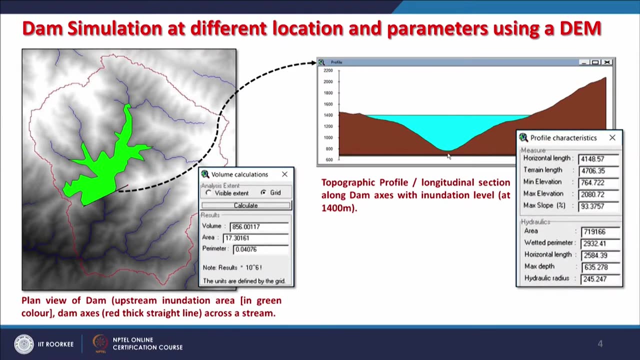 again, in this example we are having a topographic profile and it has been decided by simulation that it has to be filled up to the 1400 meter, and once we go there then we get the. these parameters- volume, area and perimeter of the reservoir- and profile characteristics are: 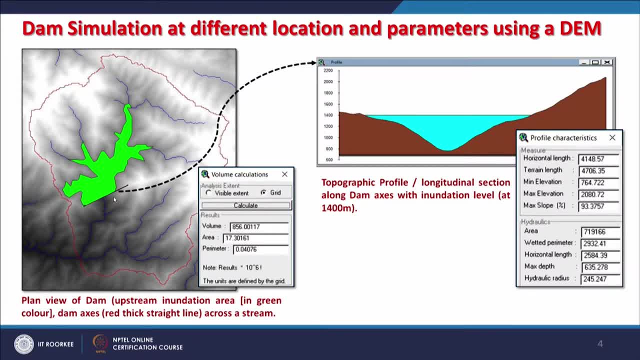 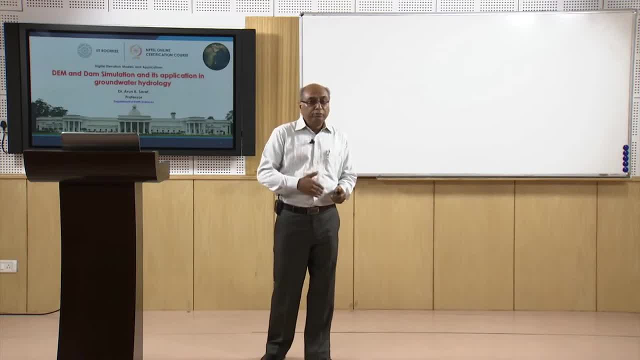 also available for at this location. If we go there then we get these parameters: volume, area and perimeter of the reservoir, and profile characteristics are also available For at this location. So that is the advantage of simulation of a dam is created there. So one can shift, you know, up stream or down stream. if we go down stream, we more water. 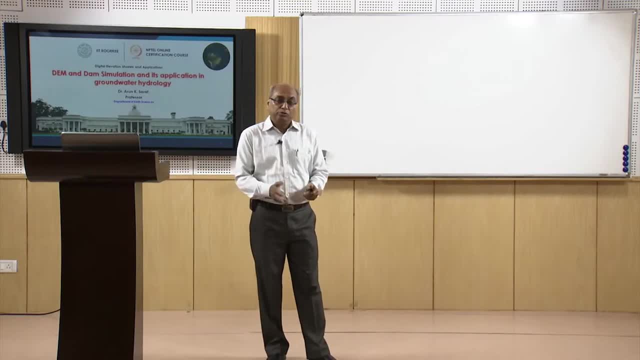 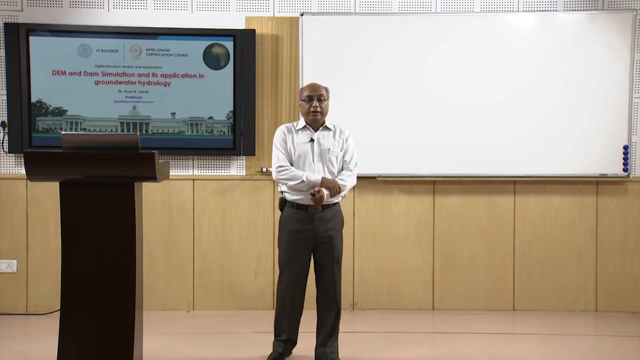 can be stored, but the height of the dam has to be changed, and so on, so forth. And this is not only for related for irrigation or hydro power, but this, this dam simulation, can also be used in groundwater recharge studies, which we will discuss a little later. 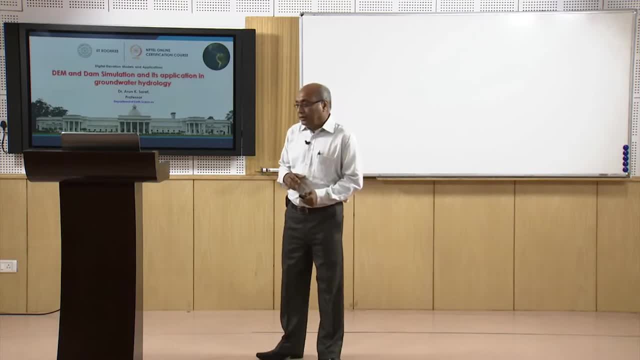 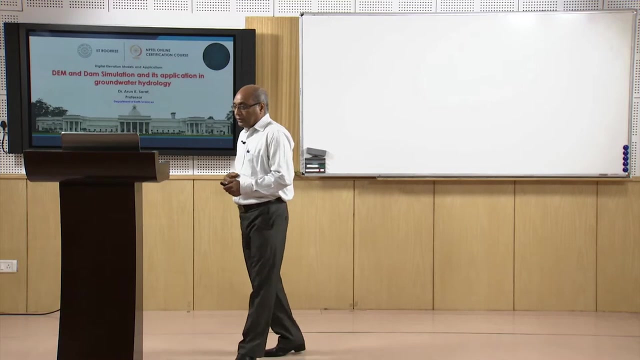 Before that, I want to bring this: how important this dam simulation studies are over a digital elevation model on a GIS platform from groundwater point of view, and how we can exploit this facility or tool of a dam simulation, which is a very important derivative of a digital 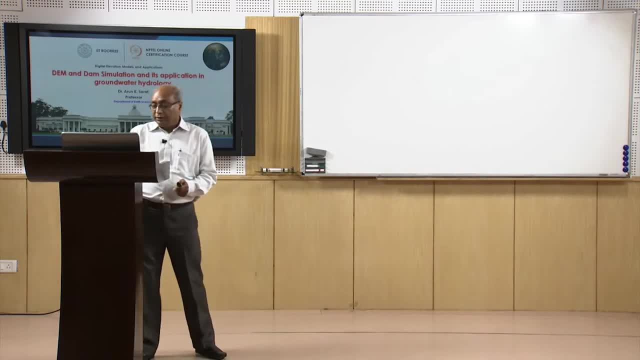 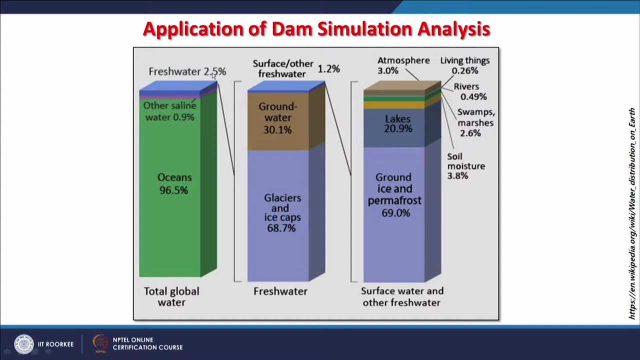 elevation model, As we know that the total global water, out of which the fresh water is just 2.5%, and that is the most precious water, because 96.5% of oceans water water is in the oceans we are having. the other saline water may be in some lakes. the fresh water is only 2.5% and 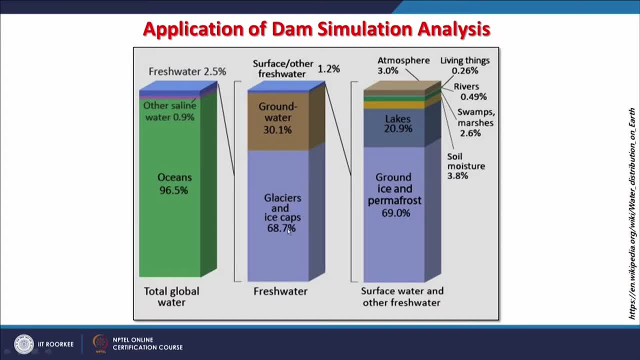 out of that 2.5%, The 68 or 67% water is available in glaciers or high caps. only the 30 or 30.1% of water is available in form of groundwater, And if we go further, then this is how the fresh water is distributed. so surface water. 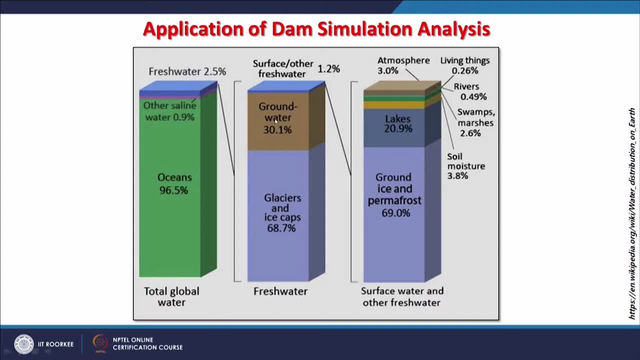 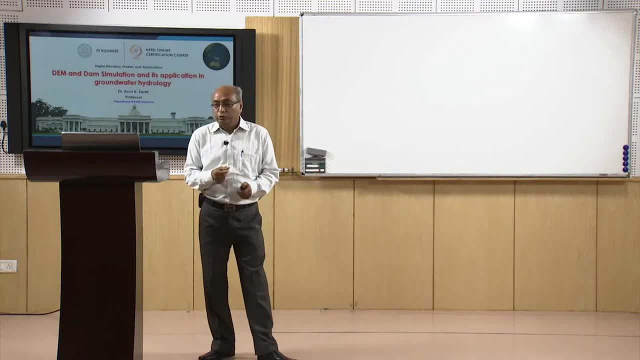 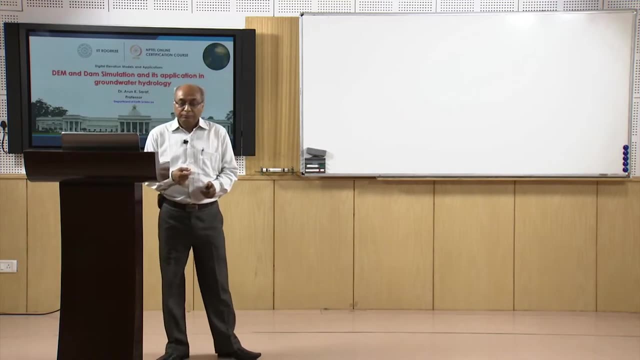 and other fresh waters are distributed. you can think that out of total 100% of water available on earth, A very tiny amount, that is only 2.5%, is fresh water and out of this 2.5%, only 30% is groundwater. 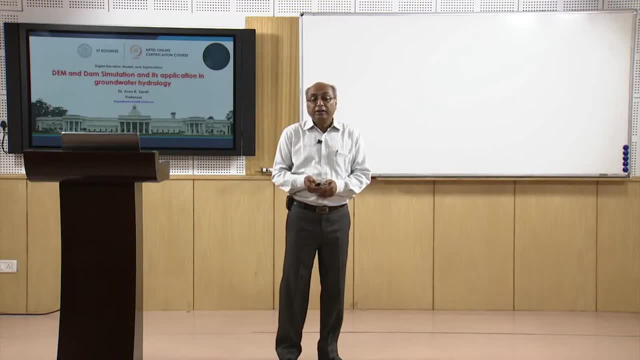 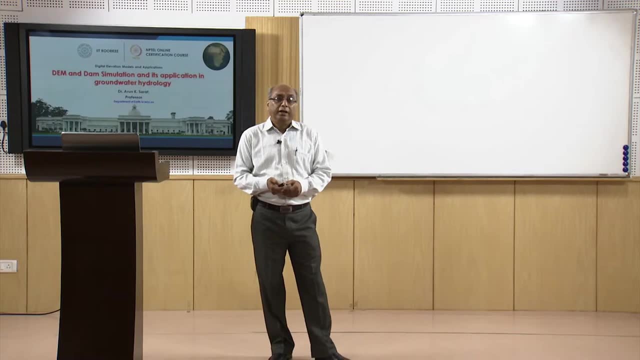 and most of the time we require this water for drinking, maybe for irrigation and other purposes. Therefore, this is very precious and has to be augmented when rain occurs. So we would like to recharge the our groundwater regime, and this dam simulation can be used. 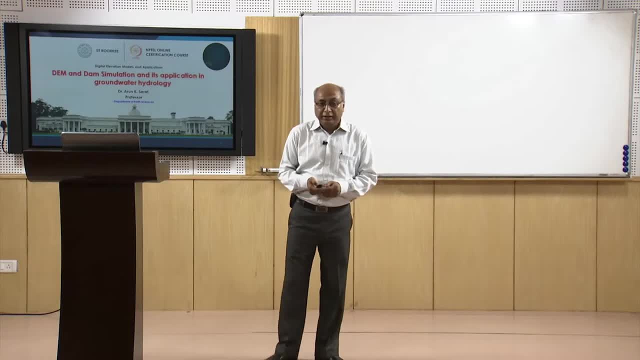 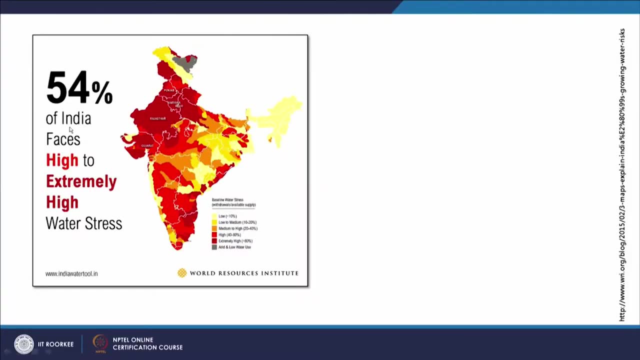 So this is what we are trying to do. So this is what we are trying to do. So this is what we are trying to do. So the plan can really help in this one. If we take India in this discussion, then 54% of India, India faces high to extreme. 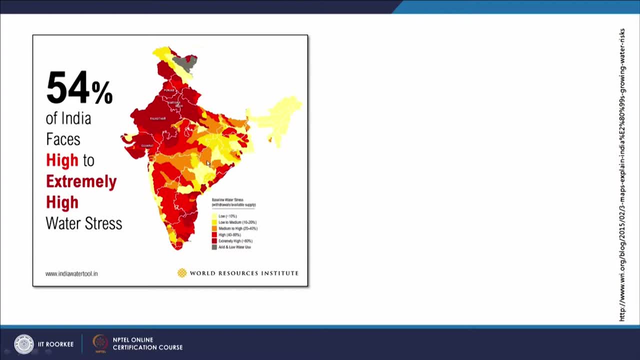 high water stresses, especially during summer months. as you can see that western part of India is having a big problem and, of course, in the, the northeast India, in eastern part, the rain is relatively much more, So the rain is relatively much more. 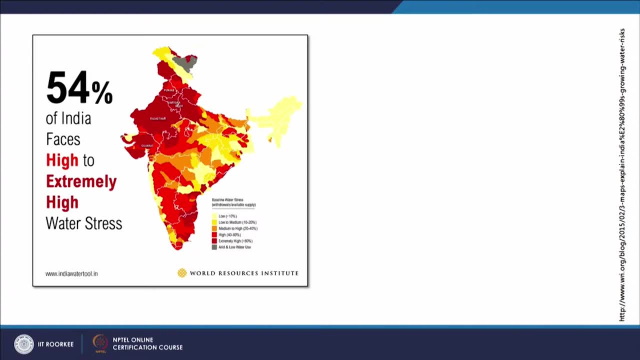 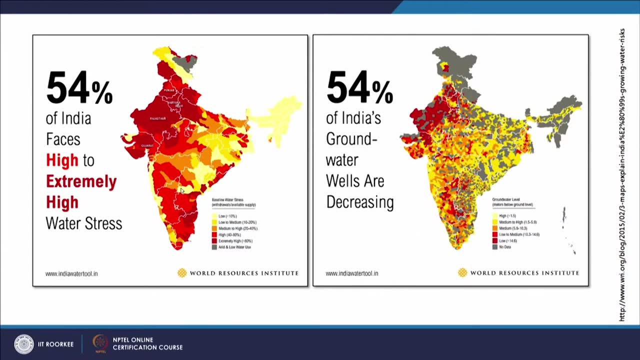 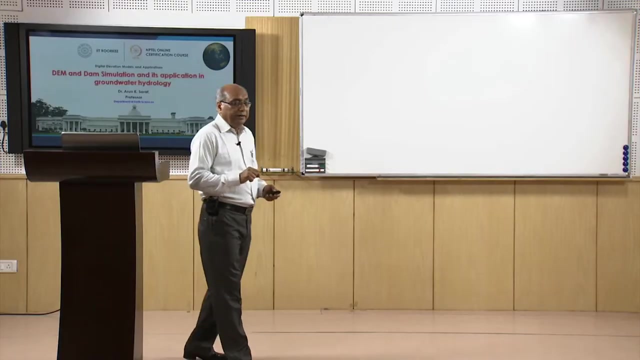 So this is somehow a natural phenomenon in India, So and it reaches sometimes earlier, so they do not have much problem compared to what the western India is having, and 50% of India's groundwater and wells are decreasing, So both percentages are same. that means that the groundwater is very, very important here. 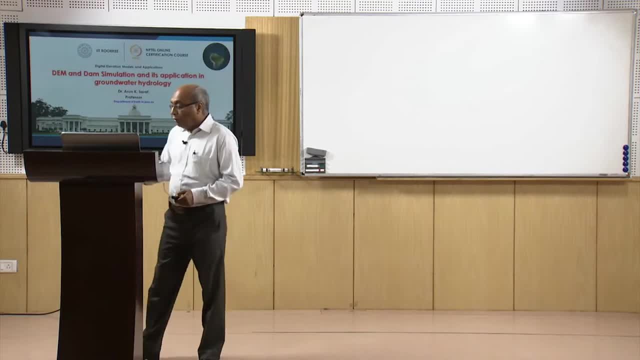 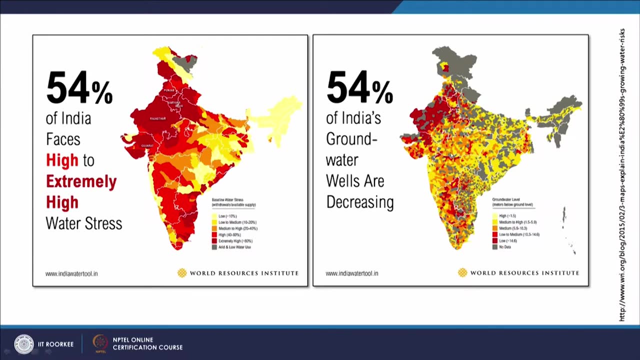 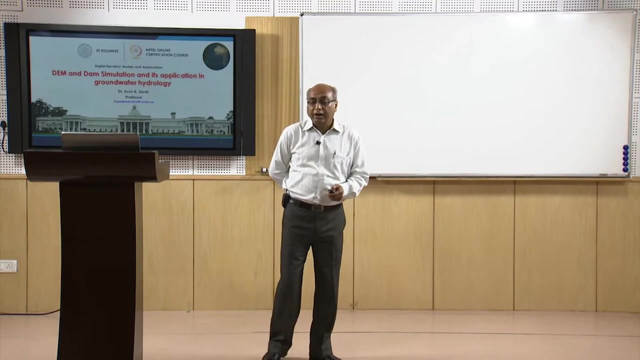 and again because the scarcity of water in the western part of India- so same is here- that the groundwater, basically water table, in these areas are also going down and down year after year. So that means the augmentation to a large scale is very much required. but the interesting 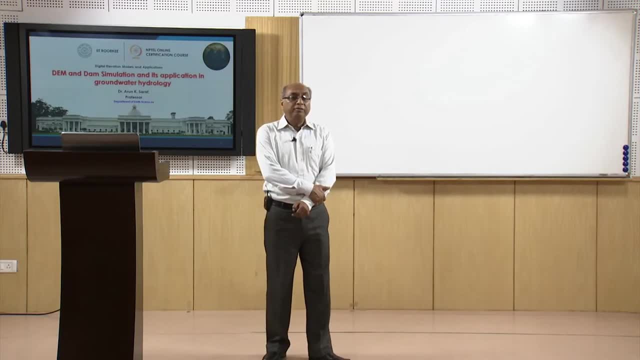 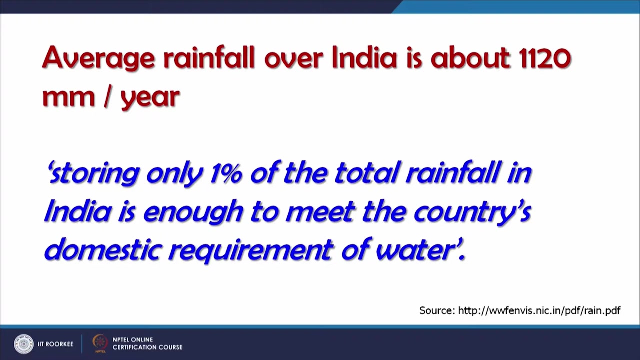 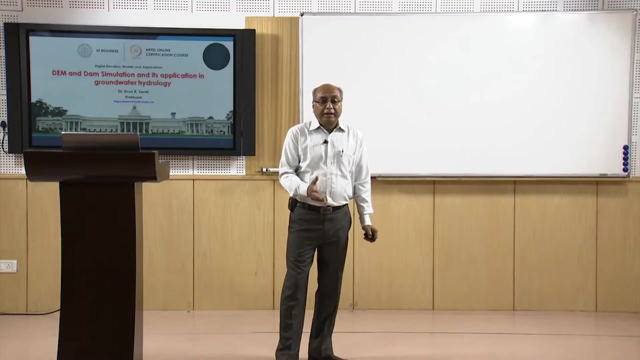 part here is that average rainfall over India Is about 1120 mm per year, which is not insignificant, which is quite good, just this. if we increase just by 1% the storage of water into the groundwater regime by groundwater recharge measures, Then the domestic requirements of water in India can be resolved very easily. 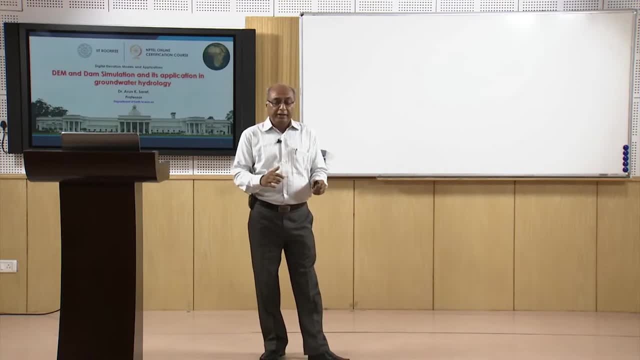 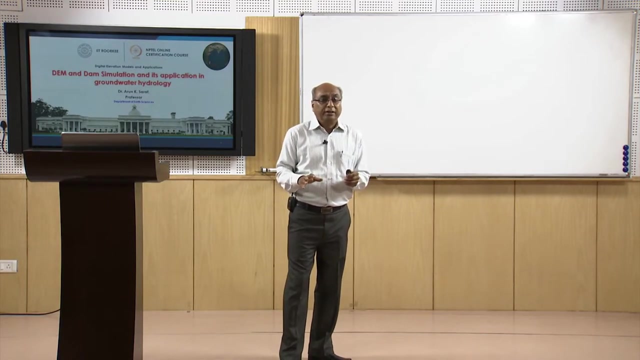 What I am trying to say is that, in average, rainfall over India is quite good, is sufficient. of course, this distribution is not uniform and if we increase the storage of groundwater by just 1%, we can resolve the groundwater problem. So the crisis which we see, or the extreme situations which we see in the western part, 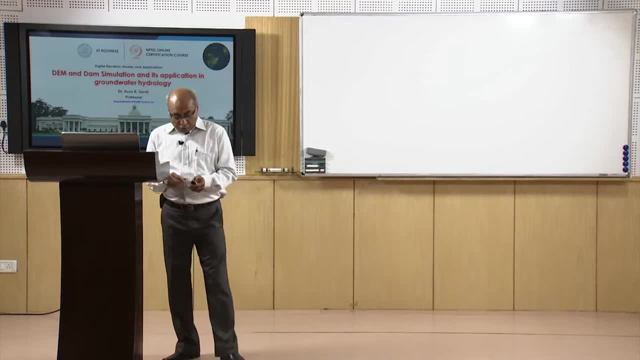 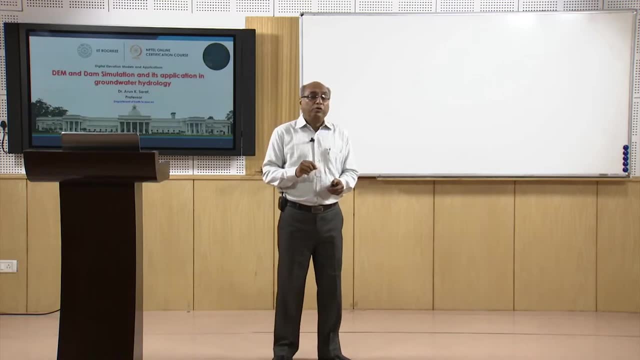 of India in terms of water stress Or in terms of lowering water table scenarios, can be resolved by just increasing 1% of our storage in terms of groundwater, and this can be done very easily by employing these small groundwater recharge structures and in where groundwater recharge structure can be constructed. 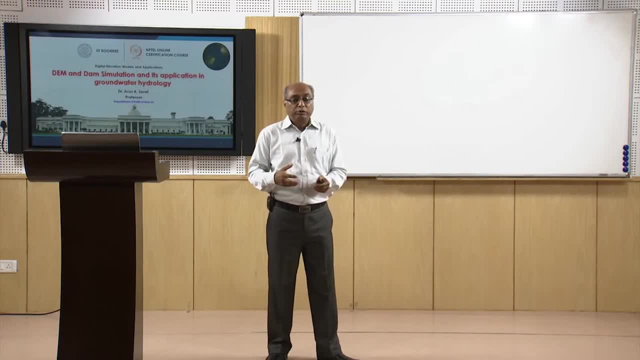 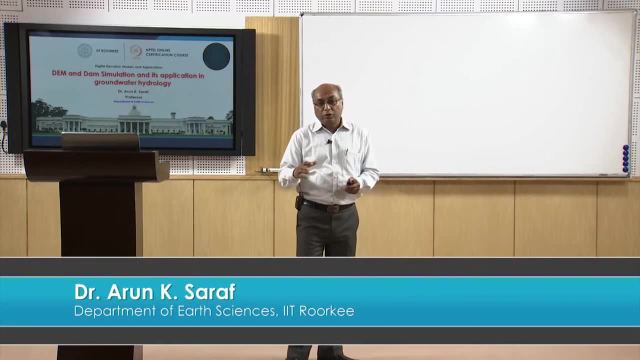 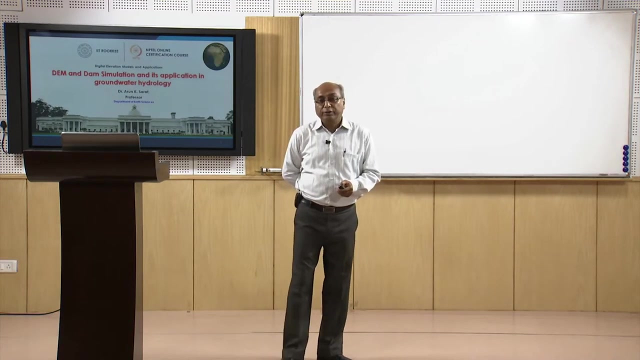 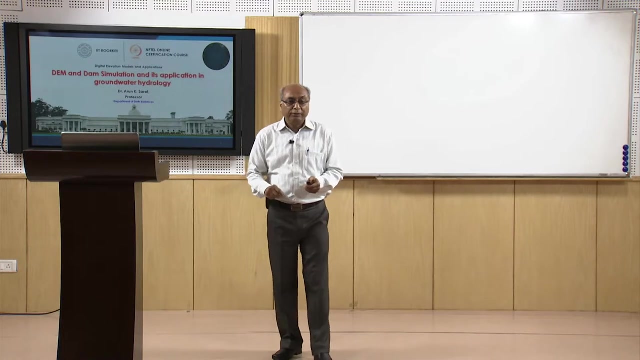 where, what would be the volume which will be stored, how it will influence all these things Can be analyzed, either based on digital elevation model, as example I have already shown, or incorporating some other information parameters which might be derived from remote sensing data. So this example we are going to see, we will focus on this one. another important information. 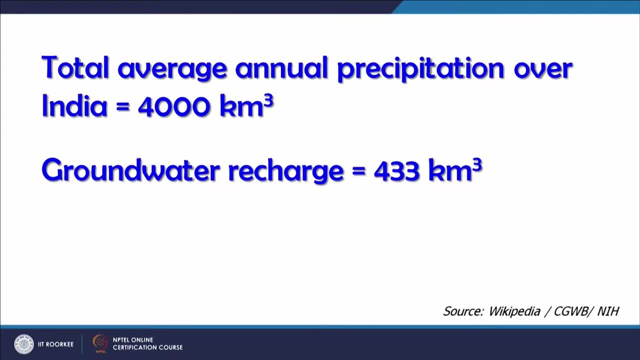 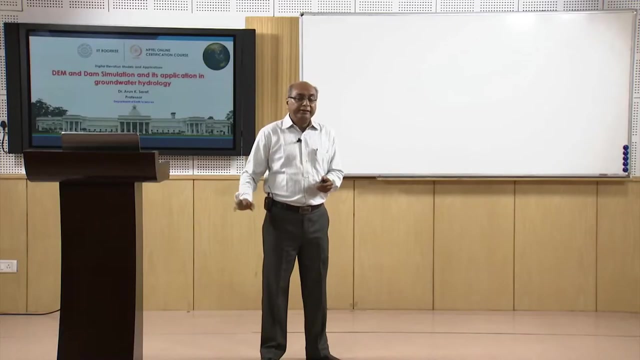 here is the total average annual precipitation over India is 4000 cubic kilometer and groundwater Ah Recharge, which is a very small amount, is going towards the groundwater, which is 433 cubic kilometer, and the most of the water is flowing as a surface runoff and ultimately ends up. 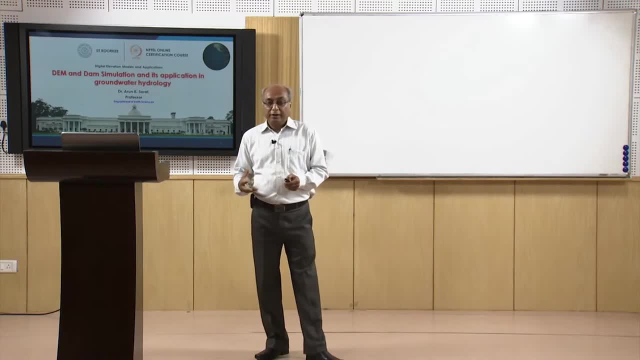 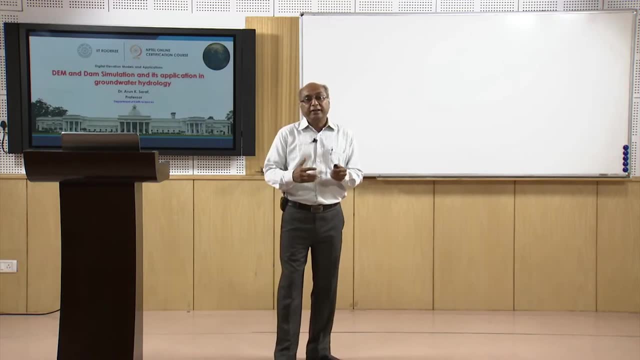 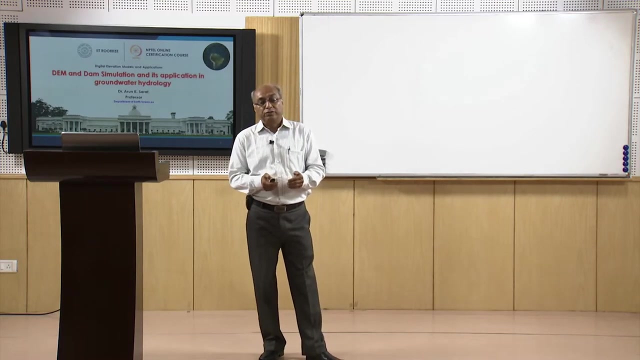 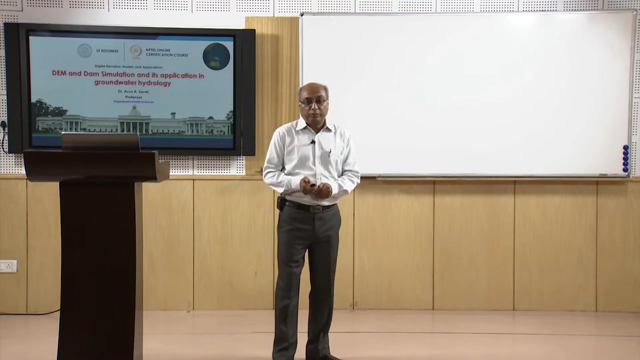 in the sea. So we need to store this water before it reaches to the sea, And first it has to be stored initially as a surface water and then let this water should go downward, Then that is world global, and So this is water locked in, because the air is much more. save the book. remote sensing. 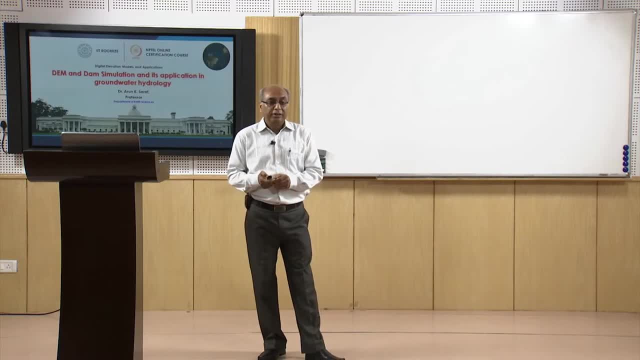 equipment by collecting water which is used in the things that you talk, amount of water to be storing all the type of water in the fresh water And the несколько countries, including India, and peace, peace, And this is 3500 cubic meter and the length water is 600 cubic meter per second. 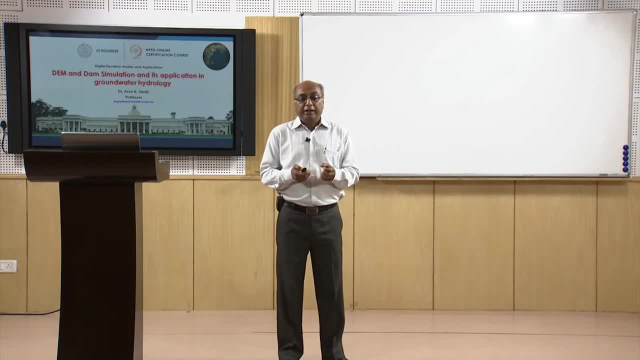 As we have imagined, the change affects how we farm. Come on, we will have to look deeper. we have seen the whole landscape here which is coming our way and the area is almost every year, especially in summer months, you are having water stresses problems. 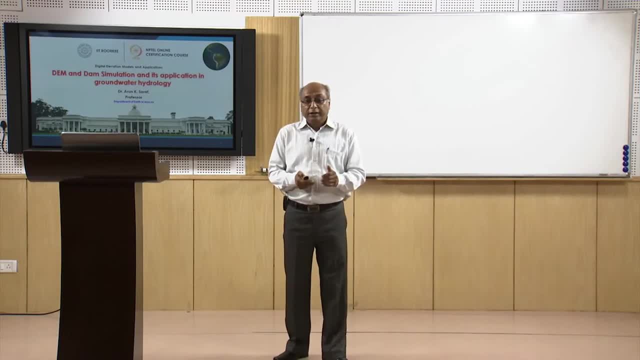 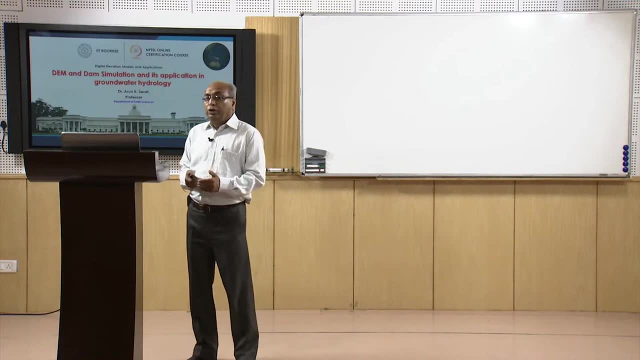 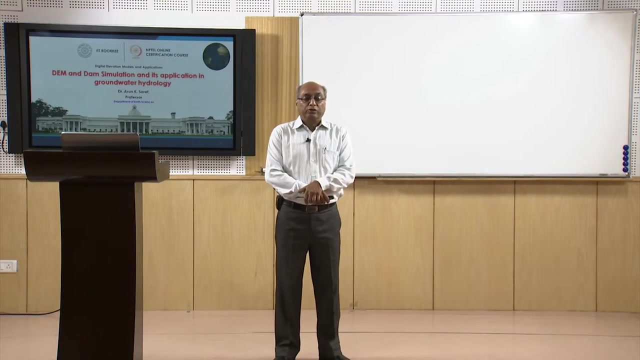 However, rainfall is about 900 millimetre per annum in this part of the country, So 900 is still not bad, but only thing we need to store the water. Example how we can learn from a simple remote sensing or satellite image and how this is. 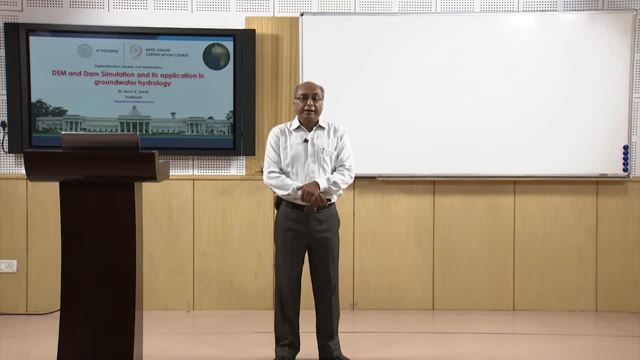 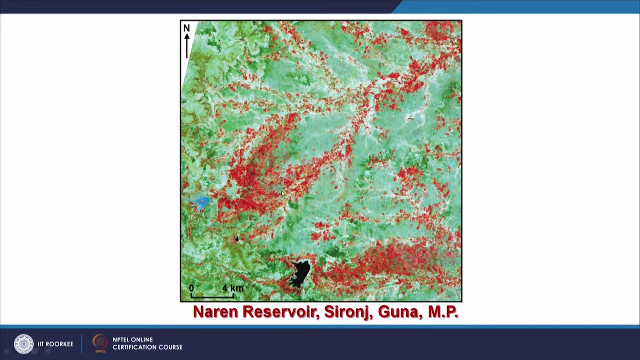 learning or knowledge we can imply on the ground while using this dam simulation technique. This is how I am going to explain quite quickly here. There are 2 dams, or rather 3 dams, which you can observe here. This is a false colour composite image in which the vegetation is appearing as in red. 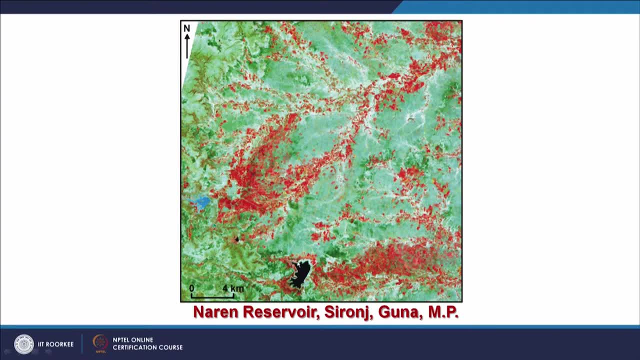 One reservoir you are seeing as a light blue colour. another reservoir you are seeing in a dark red. This is our black colour, and a very tiny one is also seen here. What you would also observe? that downstream of these reservoirs there is a growth of vegetation. 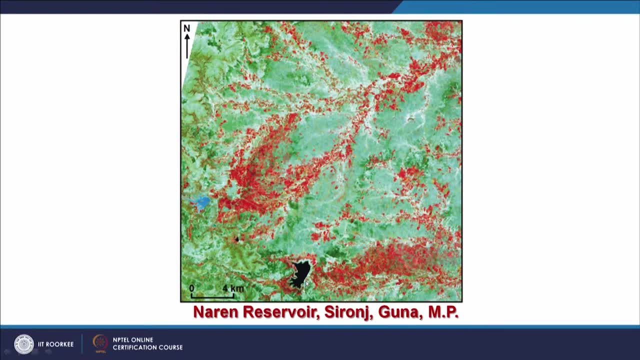 Now this growth of vegetation. this vegetation includes the agricultural lands and maybe some natural vegetation which is growing because in the downstream of these reservoirs there is a availability of groundwater and that groundwater and moisture is allowing the growth of vegetation in these areas, whereas wherever you do not have such reservoirs, like here, 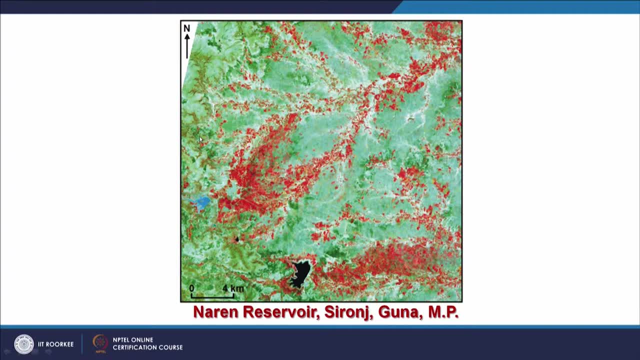 though terrain wise is same, topographically is almost same scenario. geologically these are same, different rocks and soil types are also same as here, but since we do not have any reservoirs at these margins as here, and therefore we do not have much recharge in. 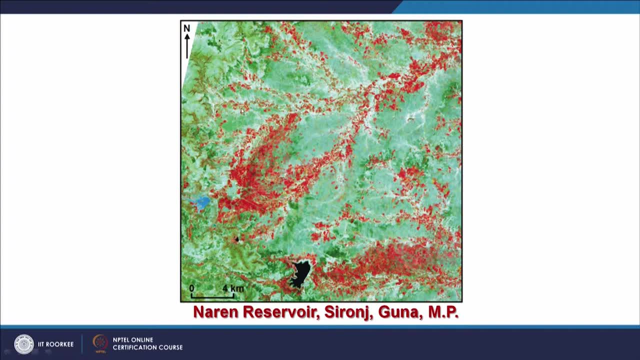 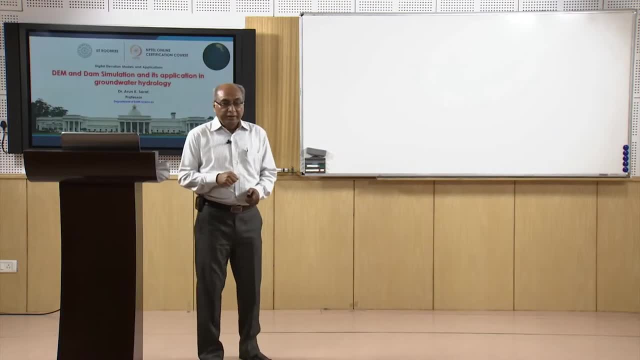 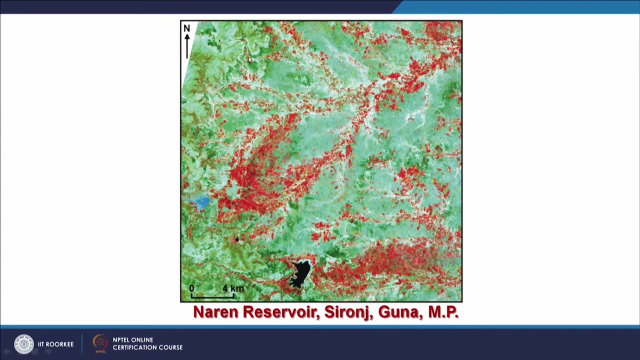 the downstream areas And you do not have much growth of vegetation. So what we learn from interpreting this, studying this particular satellite image, is that if we want to make this area green or enrich or rich from groundwater point of view, then reservoir, something like this, have to be constructed here and these will serve as a groundwater. 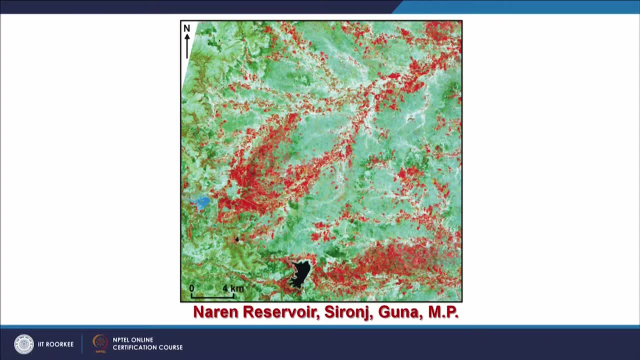 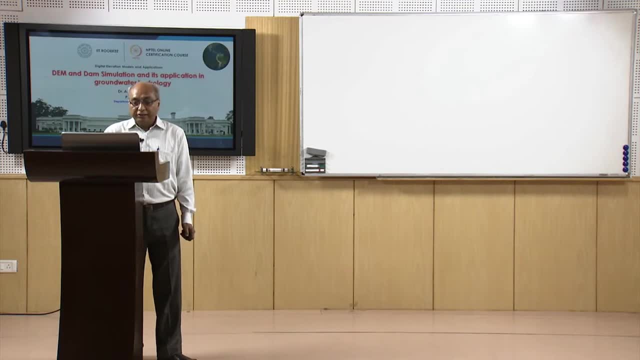 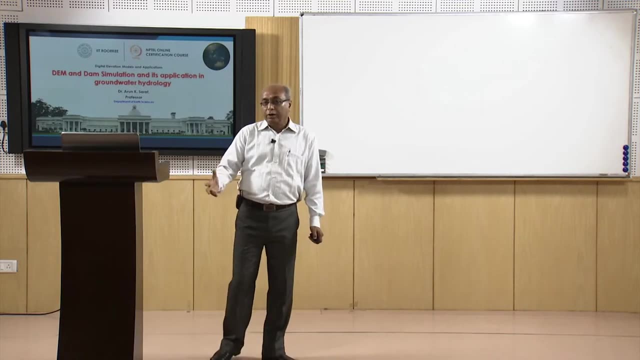 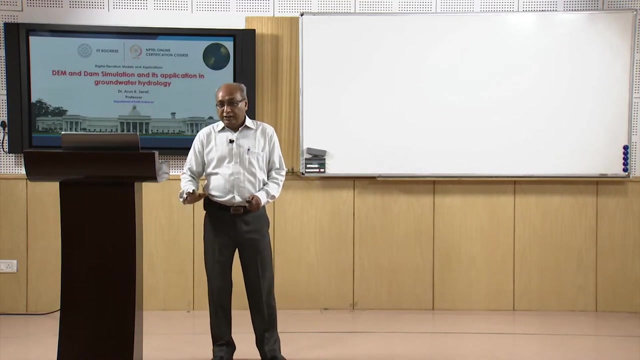 recharge structures. So what we need? A digital elevation model, Which are available, and need a dam simulation which we can simulate where exactly things will come and also we can estimate how much time it will take to recharge groundwater regime, and that can be. that can be estimated through the growth of vegetation in the same area where the same geological and topographical conditions are prevailing. So let us see, Let us see that some more differences between these 3 reservoirs, What we are seeing, that the reservoir which is named as Naren Reservoir is having the benefit area is quite large, but not as big as Sironge Reservoir. 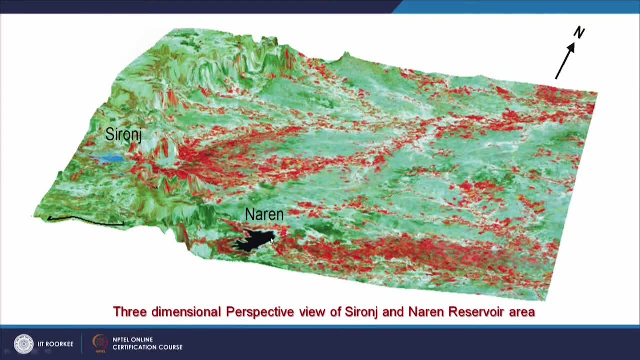 But the size of this reservoir is less as compared to Naren Reservoir. However, it is located on the higher grounds, So the hydraulic gradient Which is being provided by this Sironge Reservoir is relatively more as compared to Naren. So if we want that other parts of this area should also become green, or the groundwater. 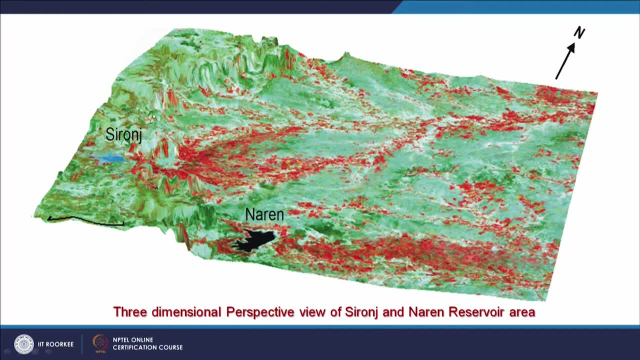 should made available, then the reservoir should be constructed at little higher levels as in case of Sironge, but not at the almost same level as in case of Naren, because this here, the hydraulic gradient, is not as big as in case of Sironge. 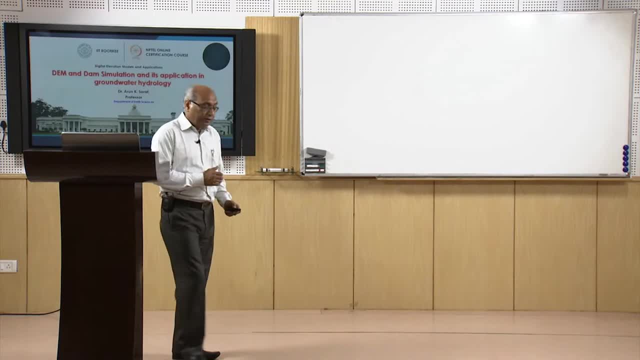 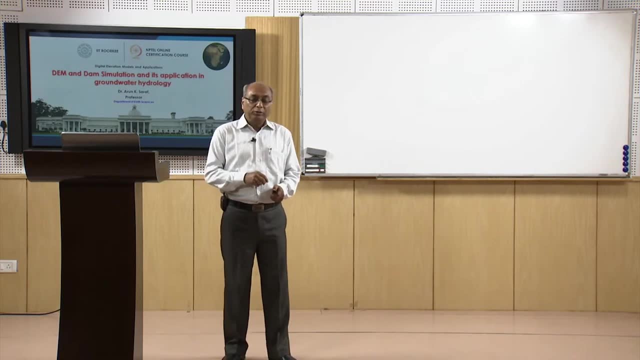 And this so just employing a digital elevation model, creating a 3D perspective view. this has given further knowledge to us that, though the reservoir may be smaller, but if it is located on higher grounds, then it will provide much better groundwater recharge than a reservoir located on lower grounds. 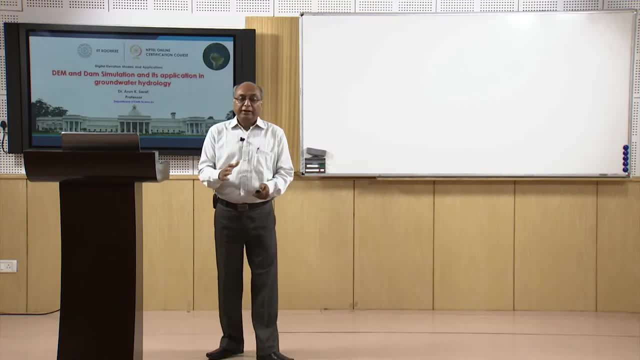 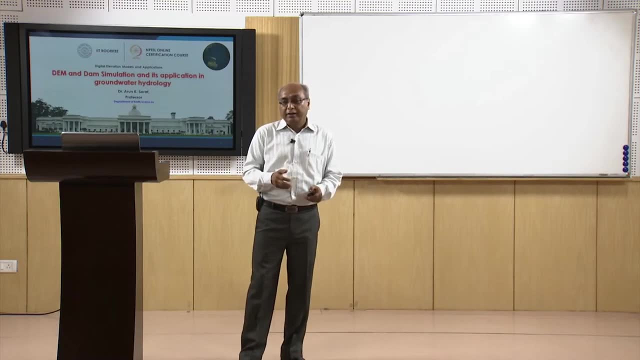 So few things which we have just learnt through the Naren Reservoir. So this is the Naren Reservoir. This is the Naren Reservoir. So the interpreting the satellite image through the interpretation of satellite image and employing a digital elevation model here, and this thing about the location of the reservoir. 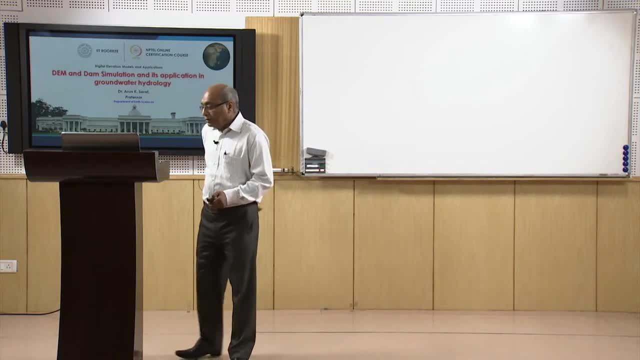 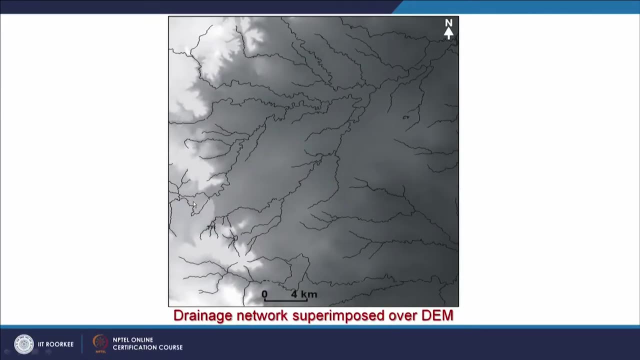 Now what? this is the digital elevation model of the same area where these 3 reservoirs are there. This is Naren, This is smaller one and this is Sironge Reservoir. what we are seeing here and, as you can see also, This is the digital elevation model that the Sironge Reservoir is located on, relatively 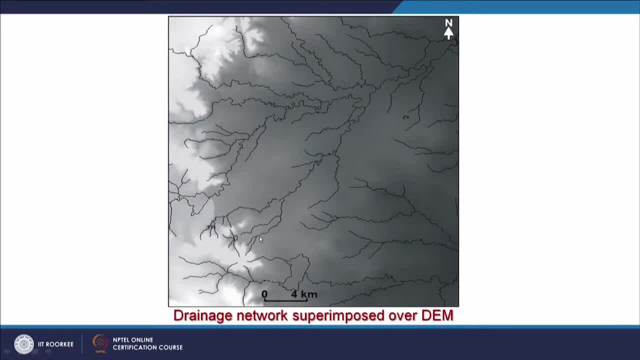 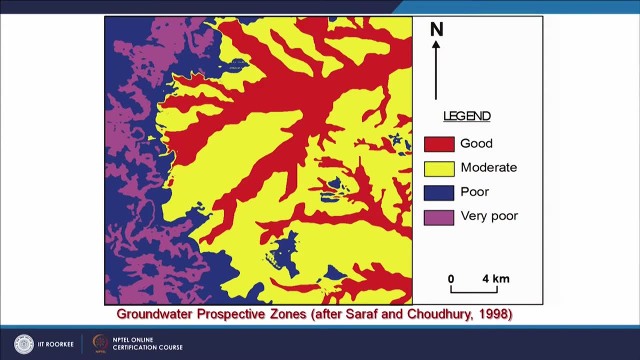 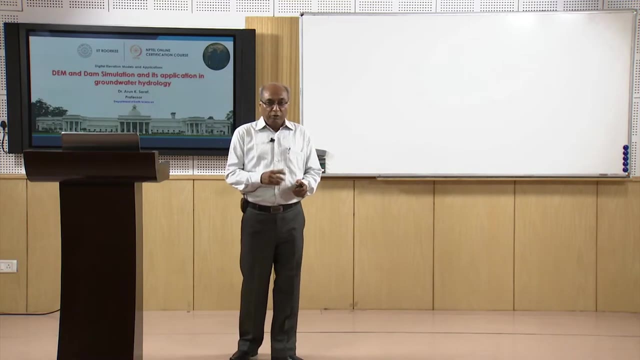 higher ground as Naren one, And, of course, it is having the Dinesh network which has been derived from this topographic sheets. So, employing these things and the knowledge which we gathered, integrating on GIS platform, including information about soil lithology and lineaments and other things, 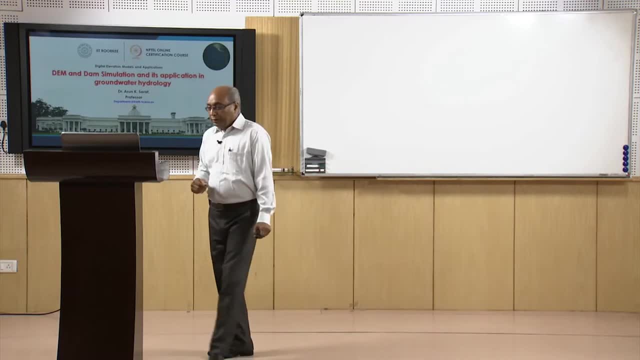 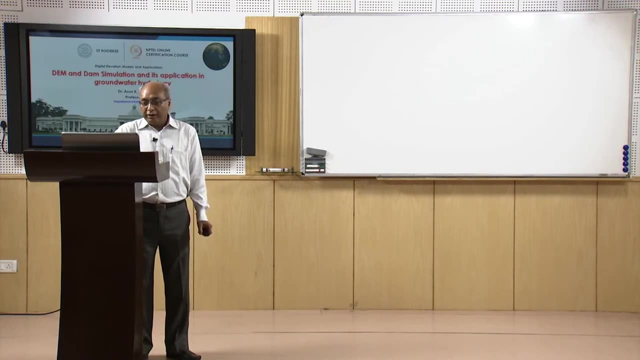 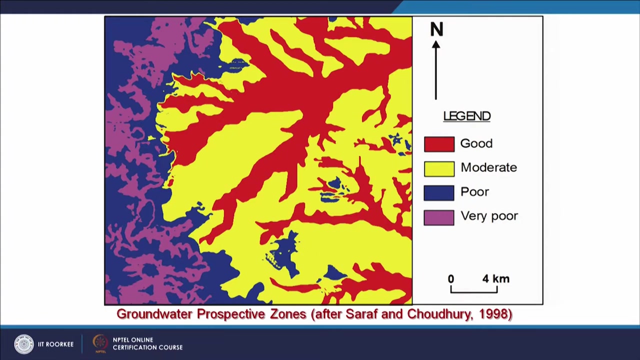 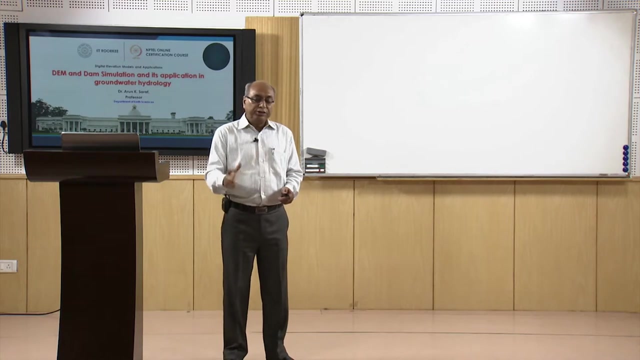 We can reach to this. So this is the Naren Reservoir. This is the digital elevation model. across the wall, there are very poor chances of availability of water. So, using a simple digital elevation model, some knowledge which has been derived or interpreted. 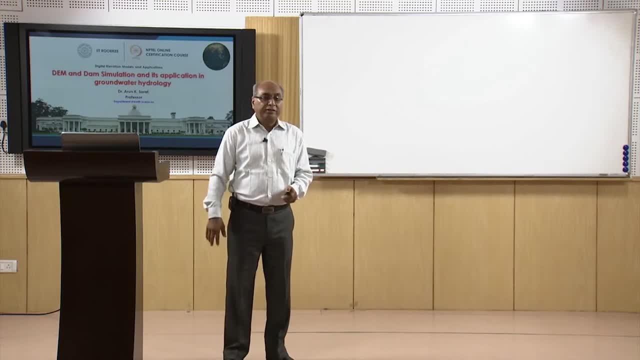 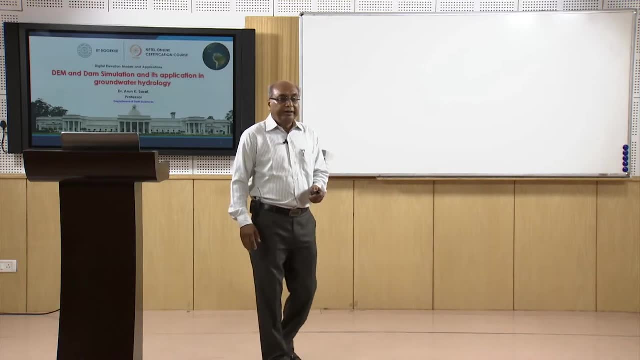 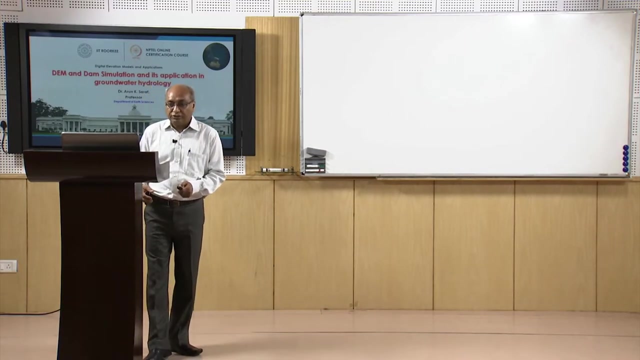 through satellite images. we can create such products which will tell us the availability of water, potential availability of water. Second thing is that which are the areas which are going to be most suitable for groundwater recharge structures, because if we have to simulate dam everywhere, one will not simulate. 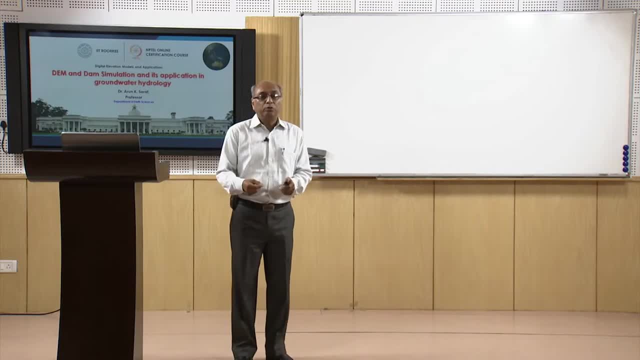 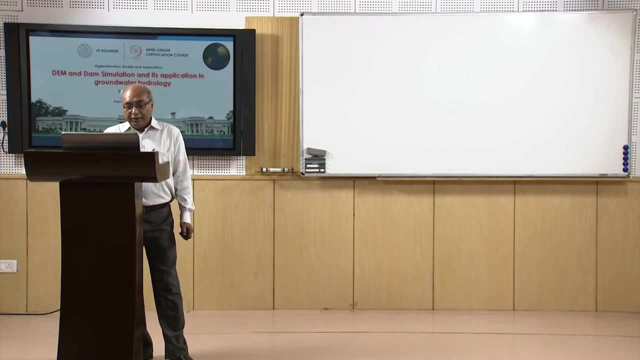 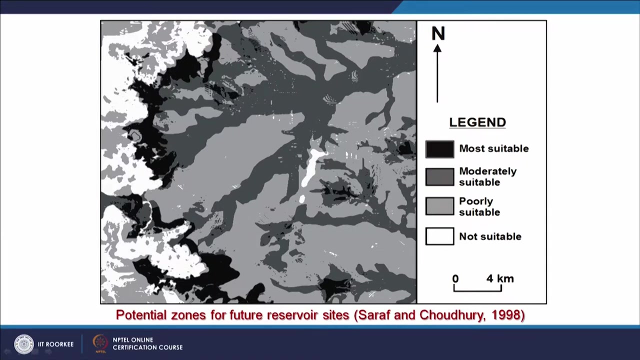 dam. So we would like to know exactly which are the most suitable areas within a study area. So in this study, again using the previous knowledge, we can generate a output that these black areas are showing the most suitable areas for groundwater recharge. These are at the higher grounds. 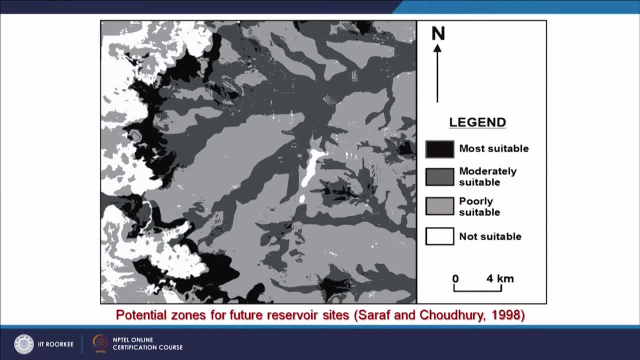 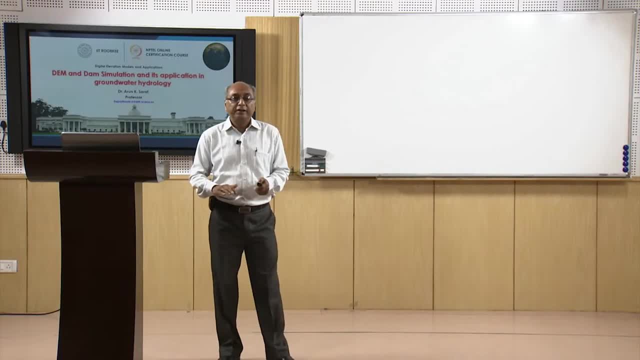 Learning from Sronge reservoir Because of better hydraulic gradient, that they should not be located on the almost same level. if we can provide a sufficient hydraulic gradient and also, at the same time, sufficient upstream catchment, If these two things can be satisfied, then these areas becomes more suitable for groundwater. 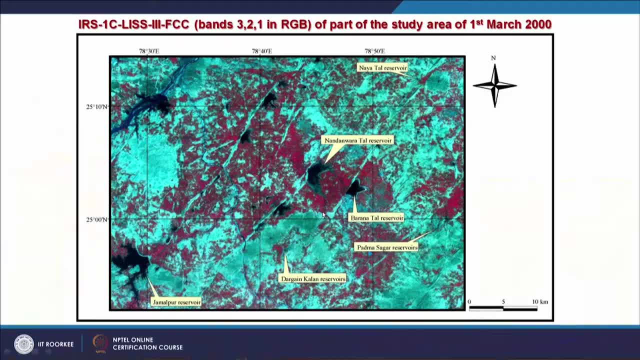 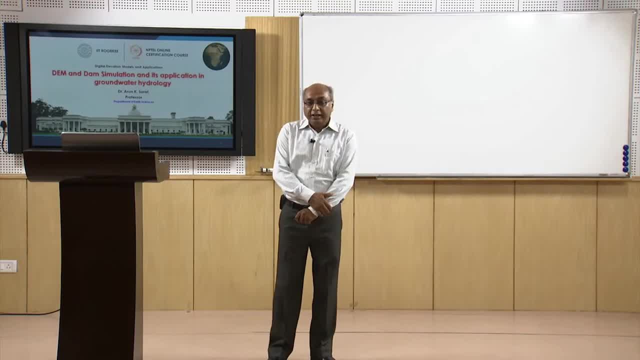 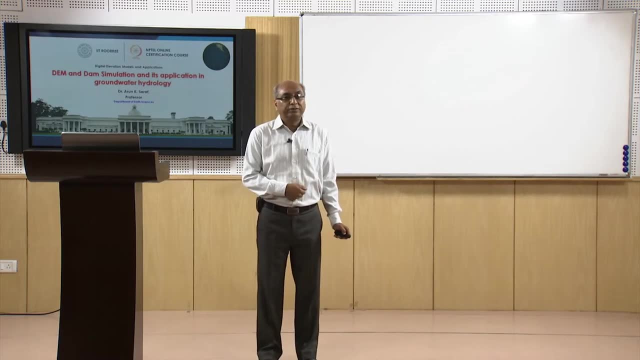 recharge. Now, further understanding one can develop, again implying satellite images of the same area. So in the case of Bundelkhand region, there are the quartz reefs which are- you can call them, as a natural dam access running for hundreds of kilometres. 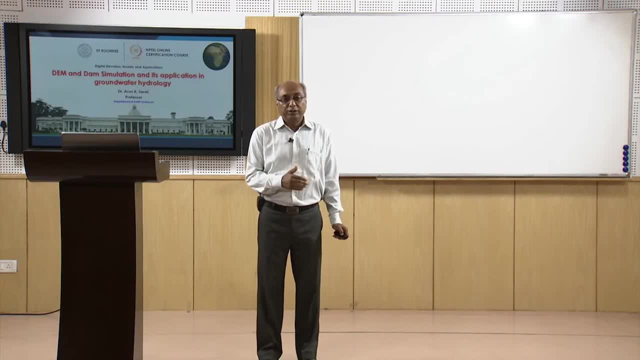 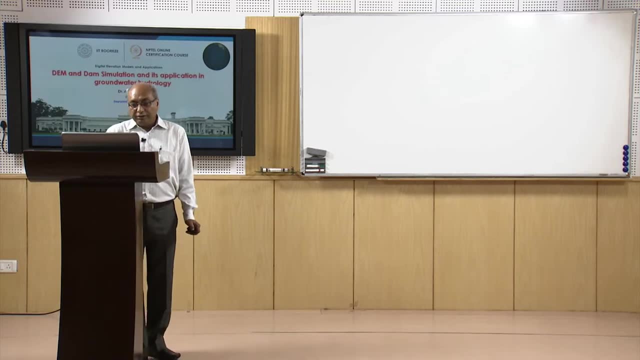 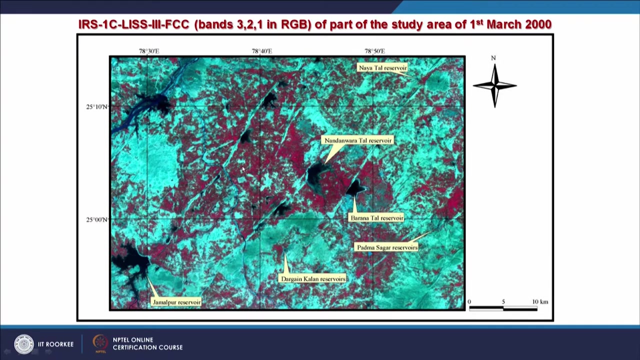 And across these quartz reefs at places you are having streams which are crossing these. So in past people knew about the advantages of these quartz reefs and they plugged these quartz reefs at places and created reservoirs, As you can see in this false colour composite. 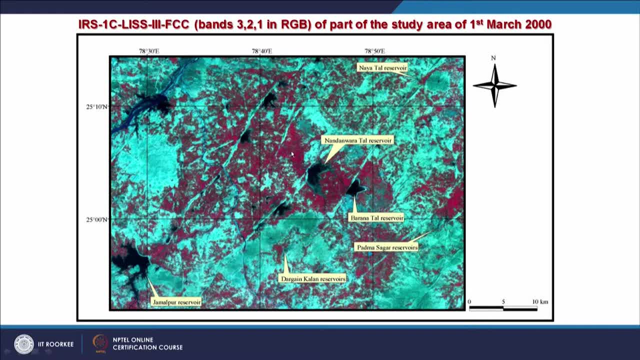 composite that wherever there are reservoirs, you see the growth of vegetation In this false colour. composite vegetation will appear as red colour and wherever you do not have reservoirs, like in this area or this area, you do not have any growth of vegetation. 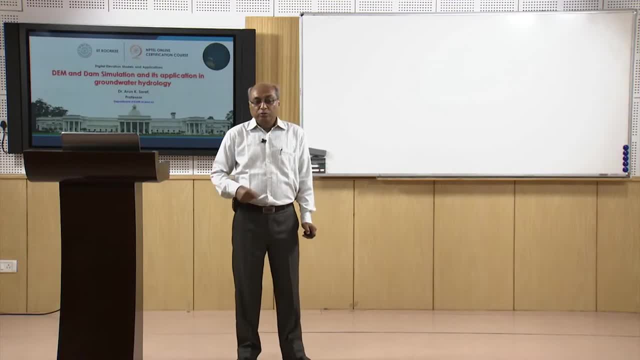 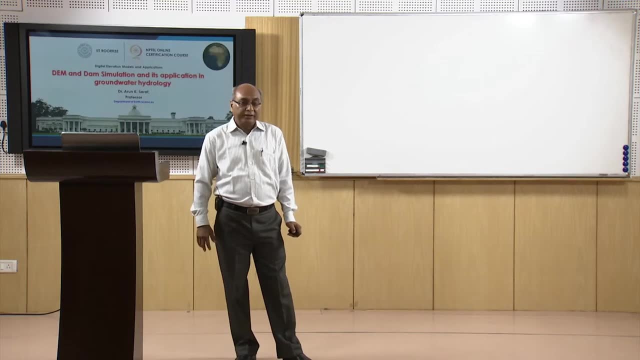 So the terrain is dry. These quartz reefs are running for hundreds of kilometres. There are still various streams which are not plugged yet, So we can plug them. imply our digital elevation model, use these DEM axes, simulate the reservoir size and we can know exactly. 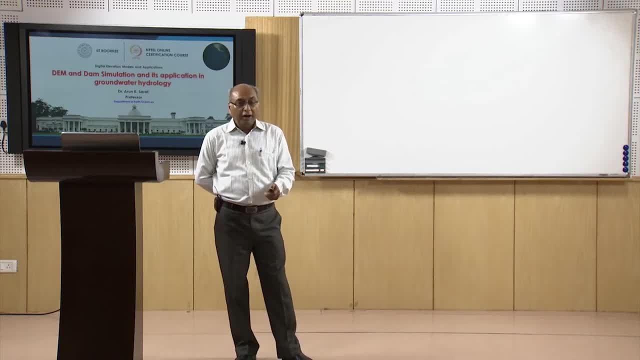 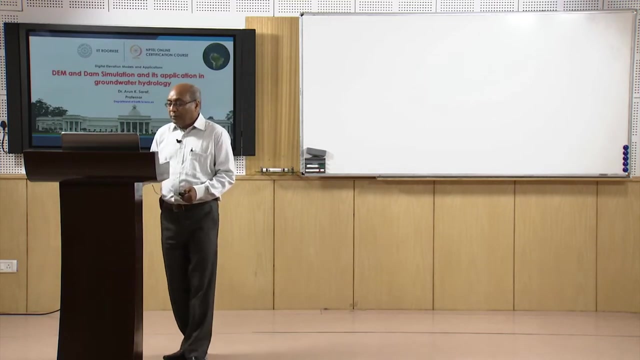 that, how much volume of water it will store, how effective it is going to be, how much time it will take to take effect for the groundwater regime. So all these things can be studied by driving a index which I will just discuss. If I take few examples of individual reservoirs, this: 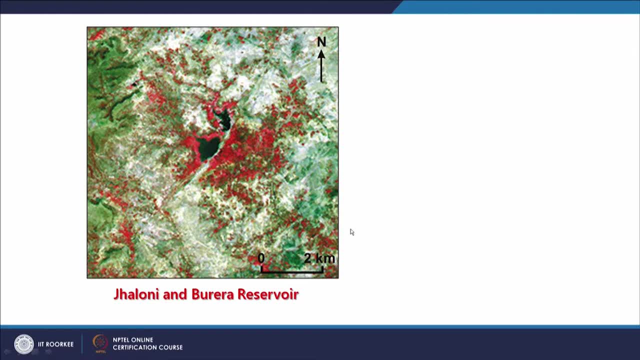 is the quartz reef and this is the downstream area. this is towards the south-east direction and the streams have been plugged, reservoirs have been created, So in the downstream area you are having growth of vegetation, as well as in the upstream- little bit upstream area. 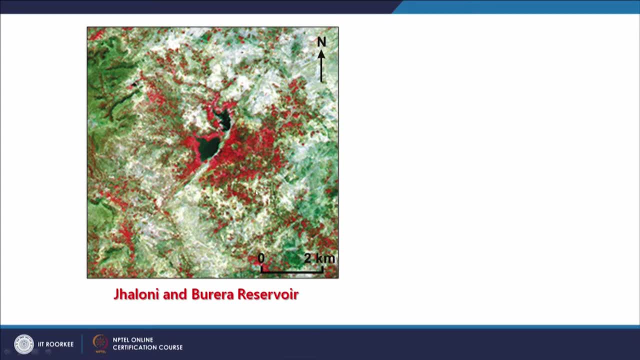 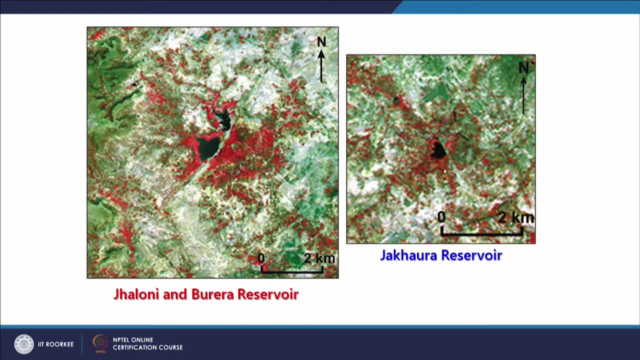 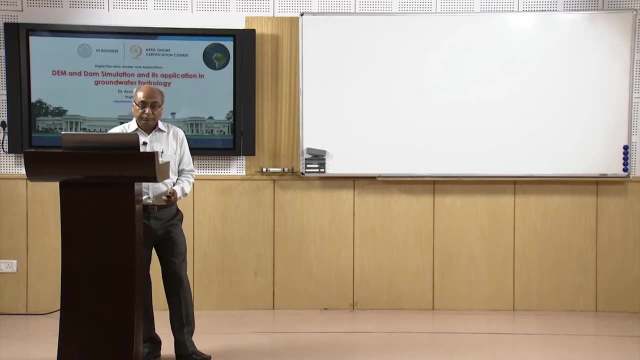 you are having growth of vegetation. Wherever you do not have the water body, you do not have any growth of vegetation. Another example here is: the downstream area is in the north-east direction and here you are having maximum growth of vegetation along this reservoir. Again, this quartz reef is. 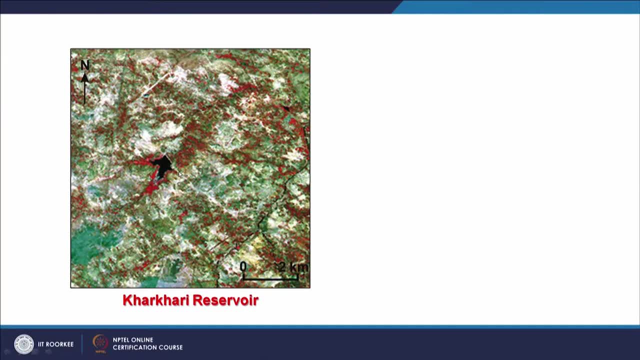 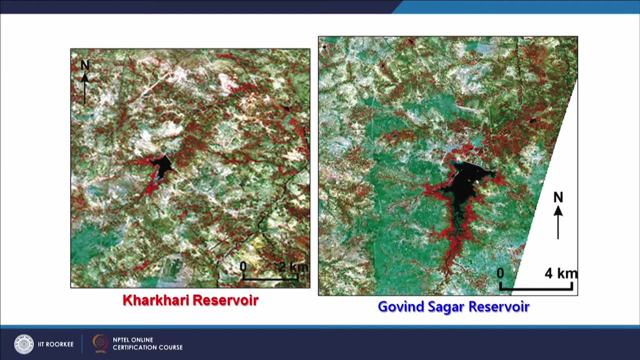 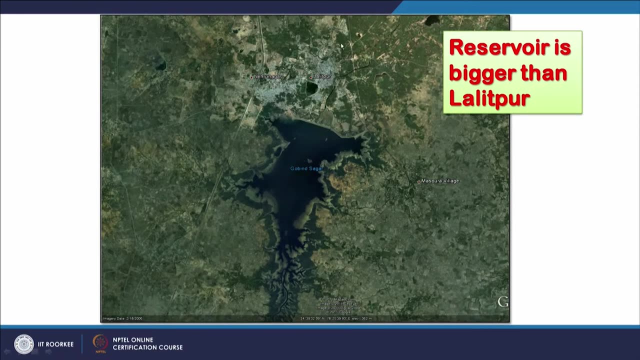 going and in downstream area you are having growth of vegetation. That is what I am calling as a benefit area. Again, one more reservoir here, which is Gobind Saur Reservoir. This is interesting. This reservoir is here. See, the size of this place is Lalitpur, which is, incidentally, my 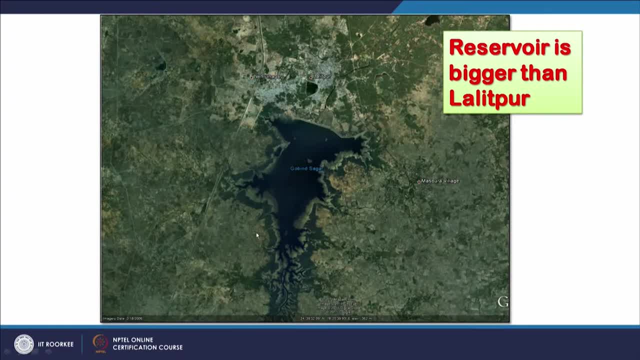 hometown and the size of the reservoir. This was constructed about 50 years back or maybe more. At that time the water supply to this small town- at that time- it was a small town- was 24 hours. But as town grew the requirements of water has increased. but our size of reservoir. 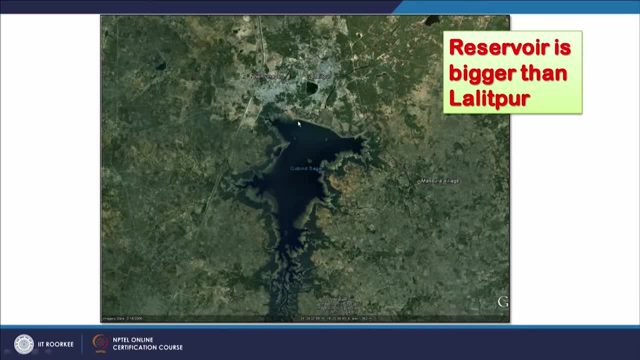 has not increased And therefore water supply reduced to roughly 2 hours per day. So that what it is telling basically that in this part of the country, when the terrain conditions are like that- hard rock terrain- then in order to supply water you need a. 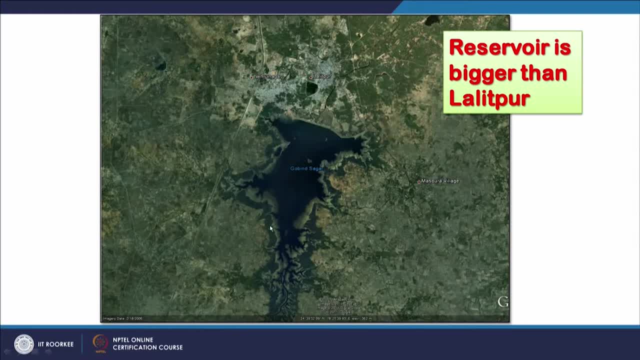 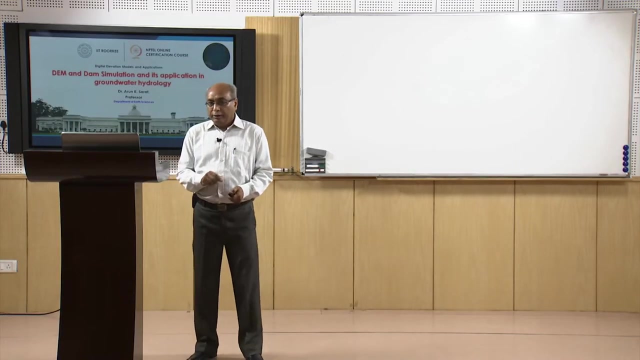 bigger reservoir, or maybe series of reservoir, maybe cascading reservoirs, to provide water, maybe 24 hours, as it was in the past. Because town is growing, Your water storage has not grown in that proportion and therefore the water scarcity is there, But at same time the rainfall is available. So if we want to drive some index or indices, 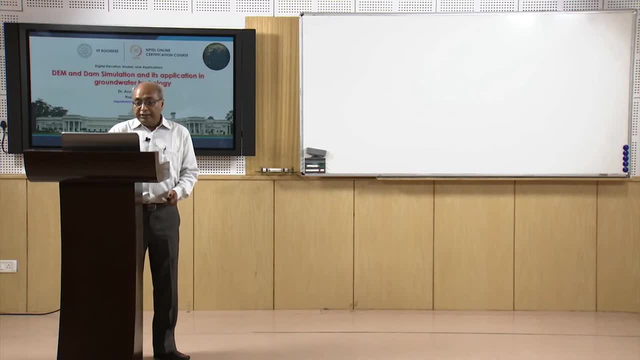 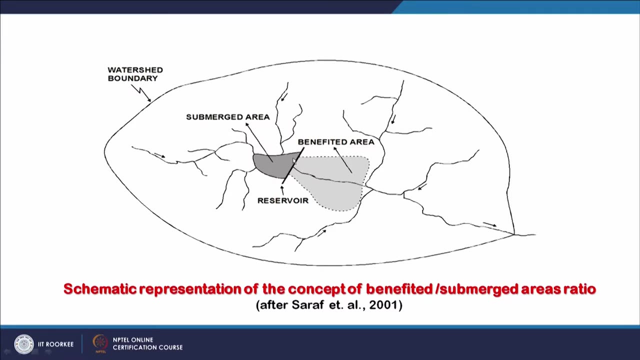 then, as I have been mentioning that, upstream of this reservoir, the dam, we can call as a submerged area and downstream of this reservoir, which we can delineate based on the growth of vegetation, we can call as a benefit area And we can create a ratio between benefit. 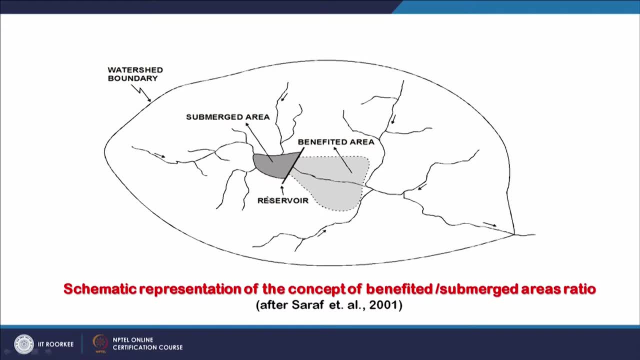 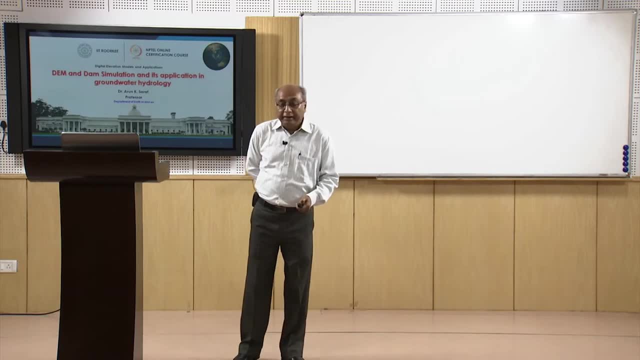 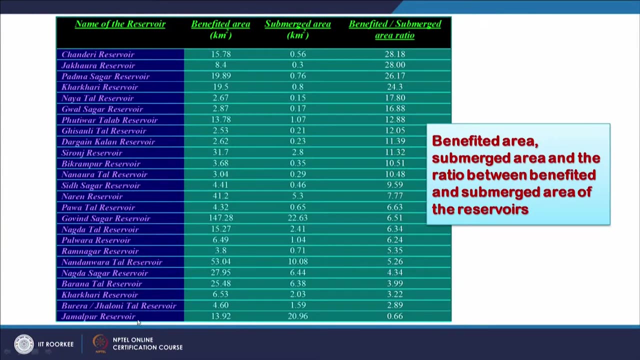 area and submerged area and can estimate, can predict that what would happen if a reservoir is constructed in that particular area. And by doing this thing and studying various these reservoirs which we are present in this hard rock terrain, we can see that, like in case, 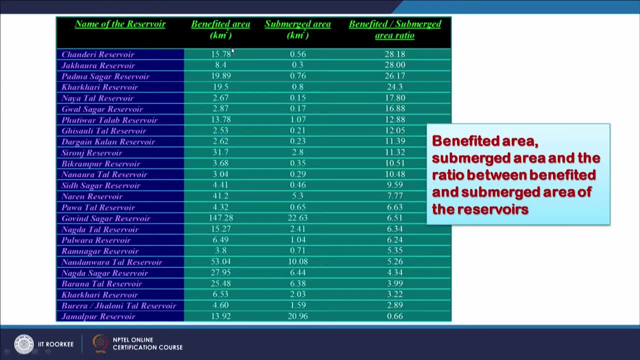 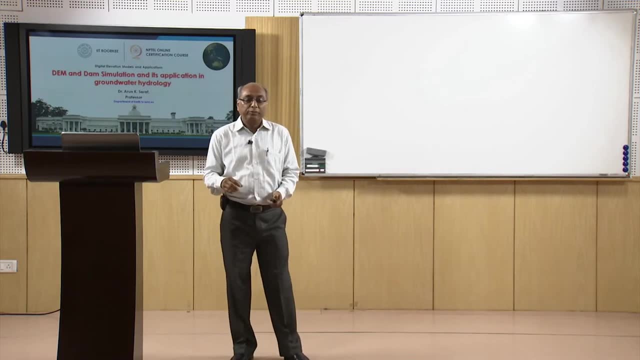 of this Chattanooga, This Chanderi reservoir- though size wise not very big, but it is providing benefits- versus submerged ratio is 28 times What it means basically, that if I submerged or invest one square kilometer of land towards the construction of reservoir in this particular area, then 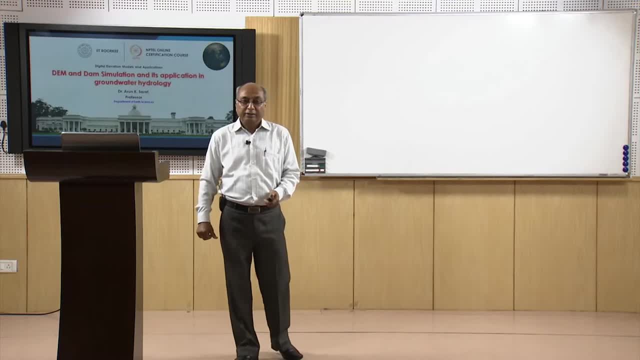 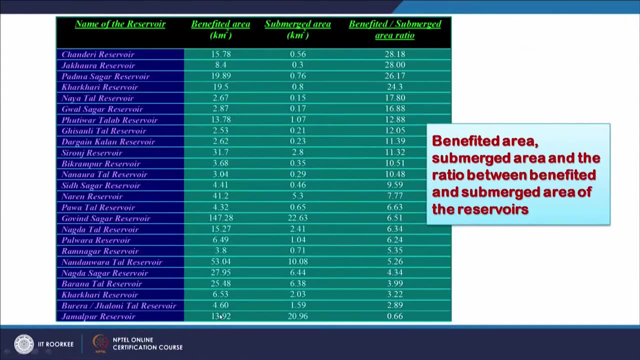 I am going to have 28 times benefit area, So my returns are going to be 28 times. It is a very good investment. However, there is one example where reverse scenario is also possible, and that this submerged area is more, benefit area is less and therefore my ratio. 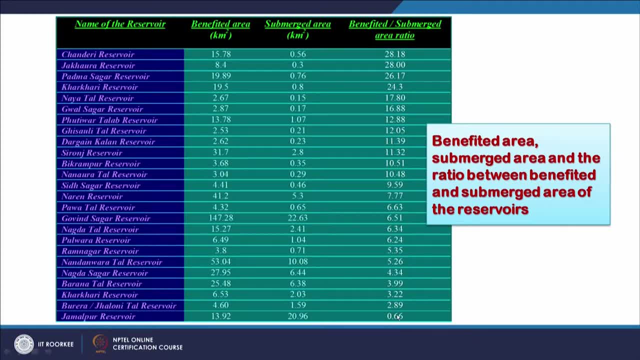 is less than 1.. So these areas may not be used immediately for the groundwater recharge or to augment the groundwater recharge, But the areas surrounding these areas where my returns are in that particular area, they are not going to be used immediately. So 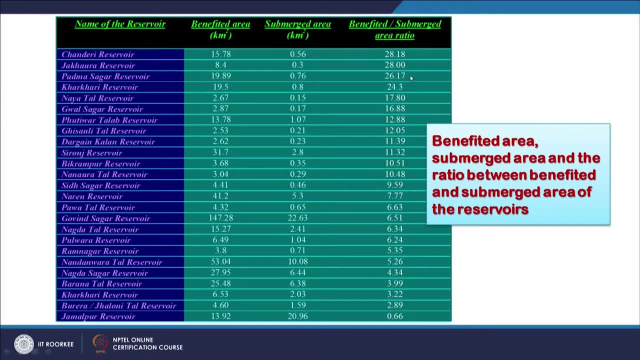 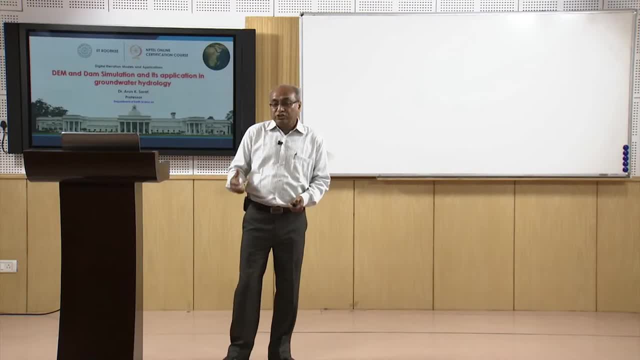 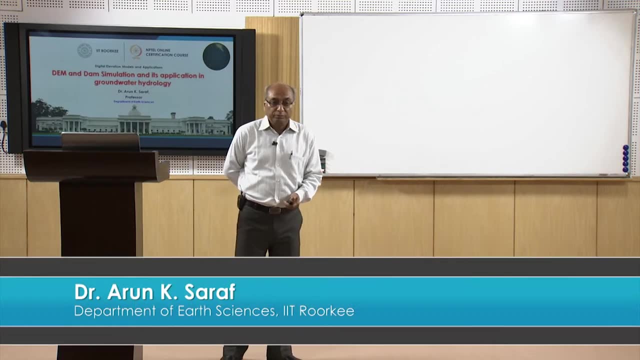 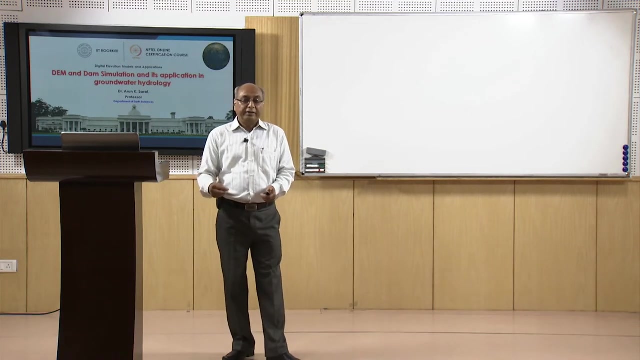 the range of 28 times, 26 times, 24 times, can be used immediately Locate where dam can be constructed and before that dam can be simulated over a dam on EGIS platform, How quickly the effect takes place and that can be reflected or measured or seen through. 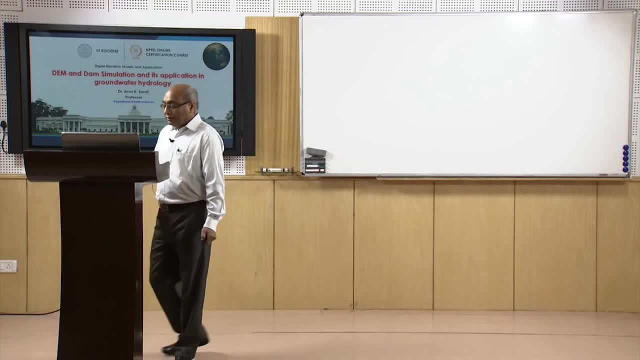 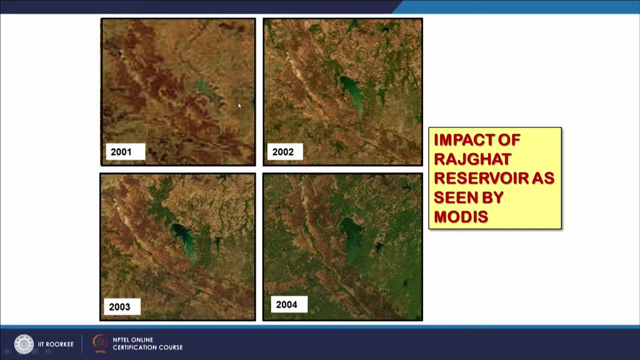 satellite images is one of the examples here. Though reservoirs are not very big, they are very large. Reservoir is larger. What we are seeing here is a 2001 image, 2002, image 2003 and 2004.. Reservoir was under construction. It was a quite big reservoir, multipurpose. 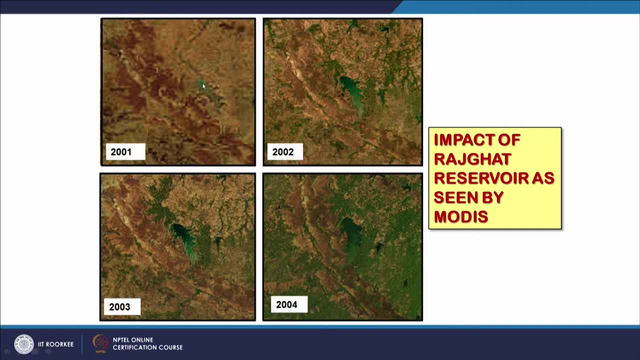 reservoir means hydropower irrigation, lift irrigation and, of course, indirectly it is providing groundwater recharge as well, as you can see here. So as reservoir was started, reservoir started filling in 2001.. This is the scenario in 2002.. 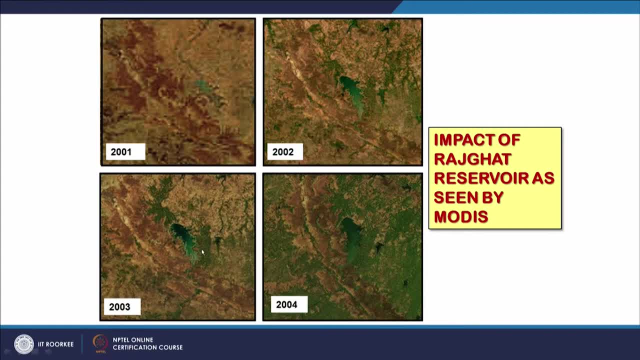 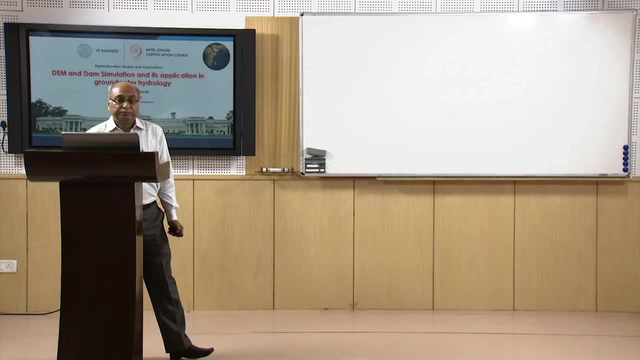 Again in 2003 and 2004,. what you start seeing? The growth of vegetation just compared to 2001 and 2003 and compared to 2001 and 2004.. So this entire area became almost green just in 3 years time, because the aquifers are unconfined here. 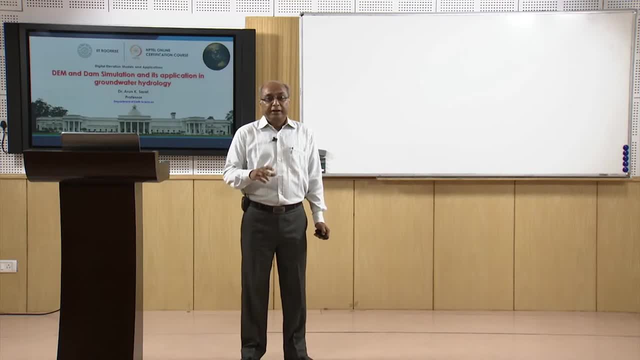 So you impound the water on the surface Because it remains mainly in the unconfined aquifers, Because these are the hard rock terrain, especially the granitic, Bundelkhand granite or Nisic complex, and only top part is having some fractures or some weather zones where 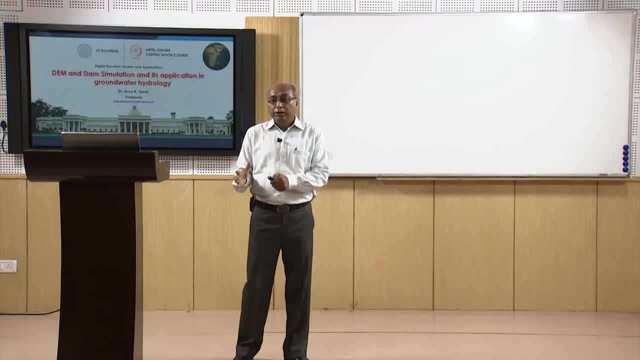 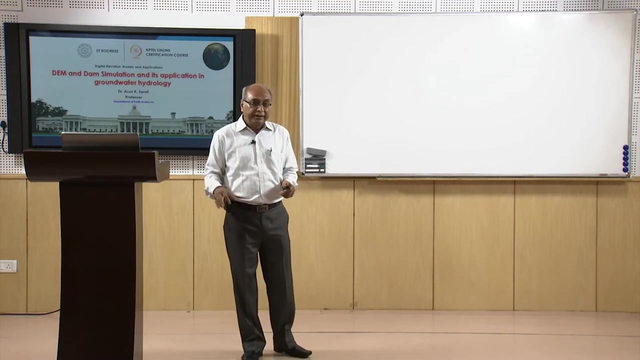 water, groundwater is stored and that is why that water does not remain very long, and few months of summer are difficult time. So if we construct reservoirs, small or large reservoirs- in that area, and then in few years time, just 2-3 years time, the effects will come. 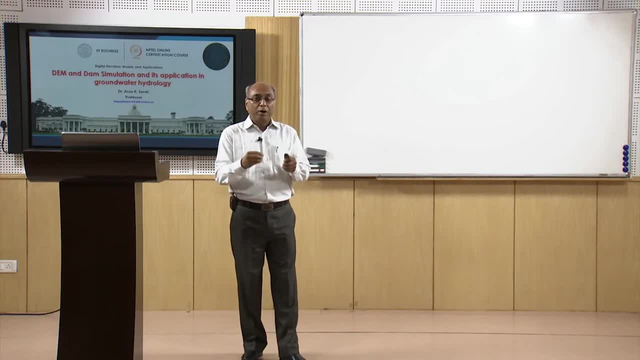 through the growth of vegetation because ultimately, when you are impounding water, it is going also towards downstream, towards the groundwater regime, recharging groundwater regime, that water is becoming available in downstream area and other parts and ultimately it is bringing growth of vegetation, Either through agriculture practices or a natural growth of vegetation. Somebody might 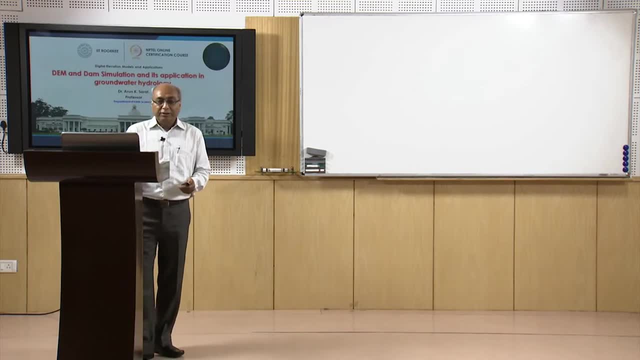 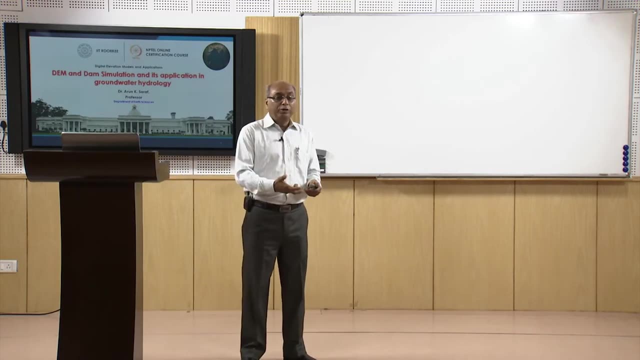 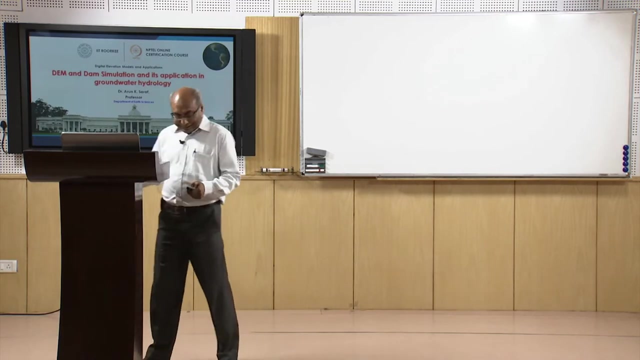 have argued with this previous slide that there might be some play, that the date or months are not constant. So 2001, which is soon, may be a pre-monsoon. 2004 might be post monsoon. So in order to clear that doubt, I have specially selected 4 images of the. 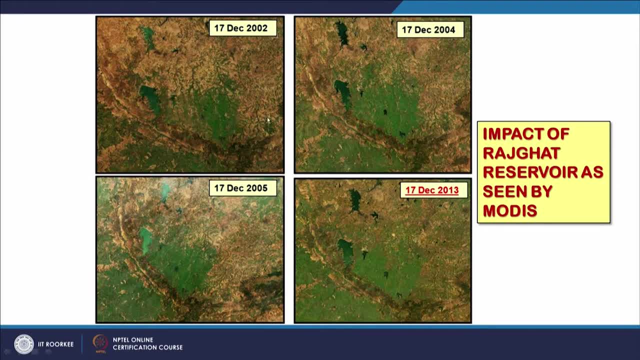 same date of different years which were cloud free and, as you can see that in 2002, this reservoir got completely filled and this is the effect that in 2013,- this is the scenario. Just compare 2002.. So this time series remote sensing data can allow us to know that. how? 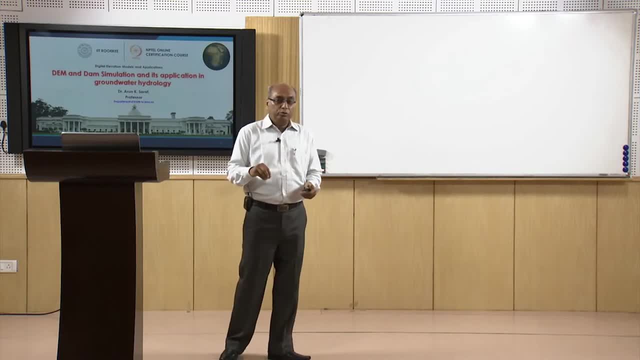 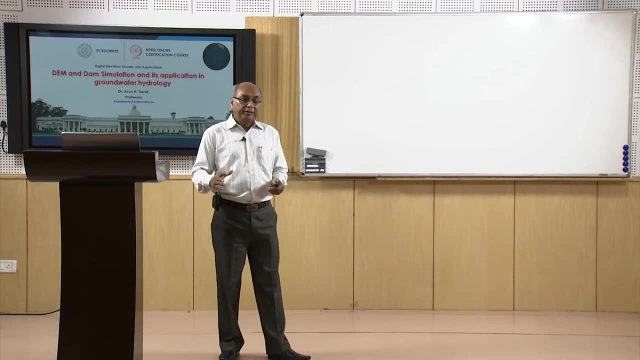 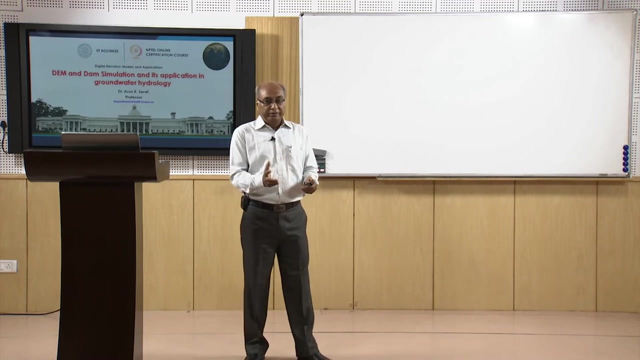 much time I would take to get this benefit in a particular area. So you know that one way is investment of the land. that is the ratio benefit versus some much, and here is the time also can also be estimated how much time I would get the returns. So how much return I can estimate. 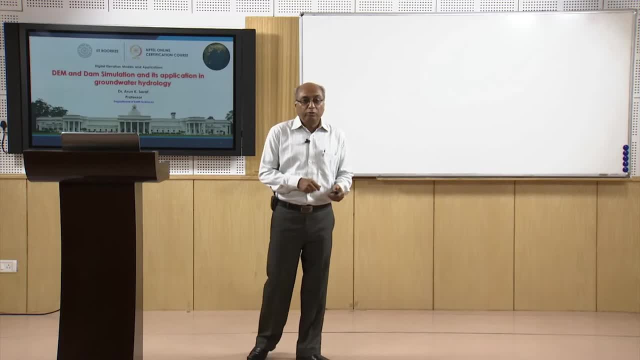 how much time it will require to get those kind of returns. So how much return I can estimate. how much time it will require to get those kind of returns. So how much return I can estimate. how much time it will require to get those kind of returns can also be estimated. 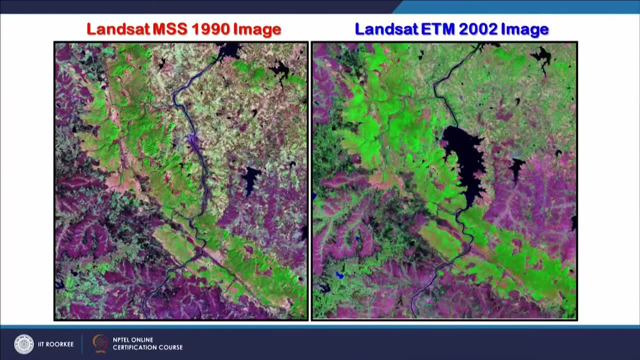 here. Same example here: that in the year 1990, this was the scenario- and in the year 2002, this is the So. in 1990, there were no signs of this reservoir, the Rajghat Dam or Rani. 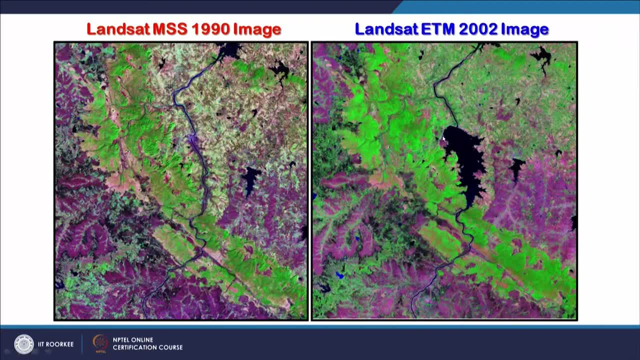 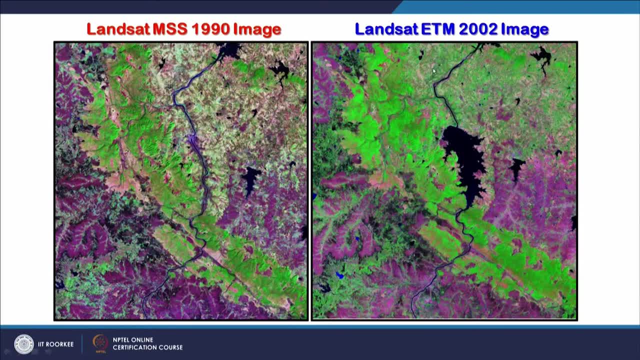 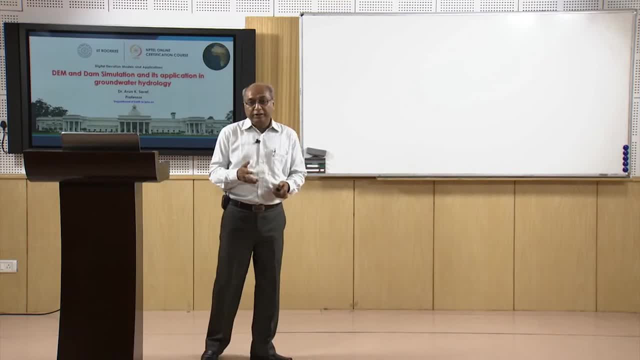 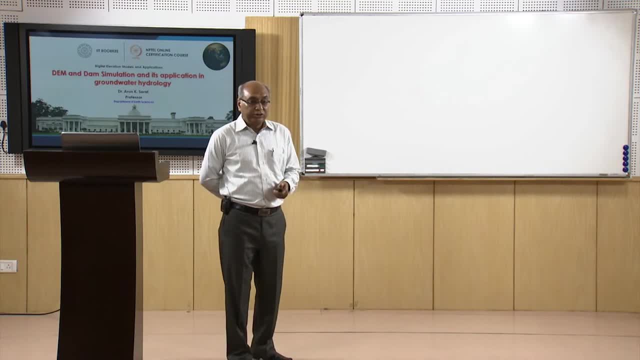 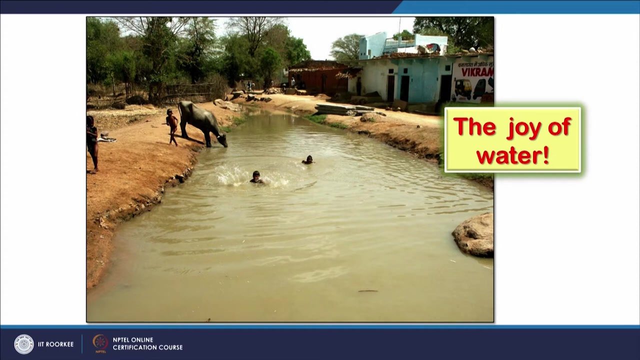 through lift irrigation and, of course, groundwater recharge, as you can see here. And this is the benefit of water. This is the joy of water in the area where water was scarce, But because of construction of these reservoirs and especially these canals, which are completely 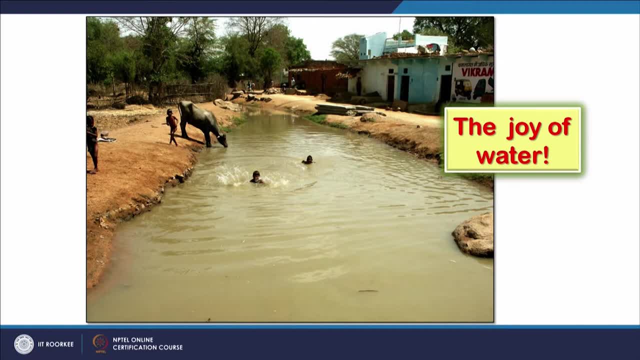 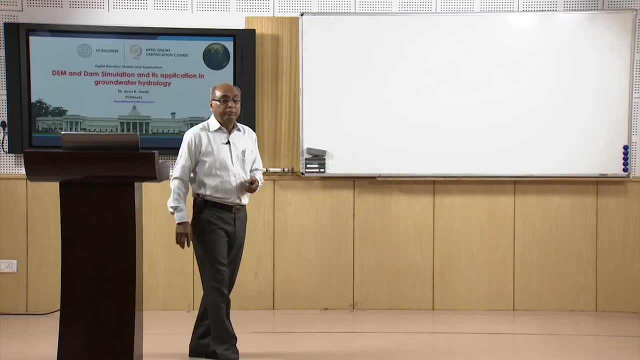 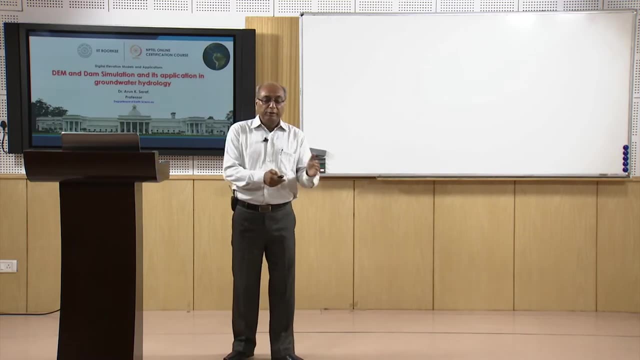 unlined canals. they are recharging the groundwater regime. As you can see in the surroundings you are having growth of vegetation. In just few years time you will have vegetation growing all over the area. Now I take again- we go back to that dam simulation- How exactly we can now exploit that tool, or 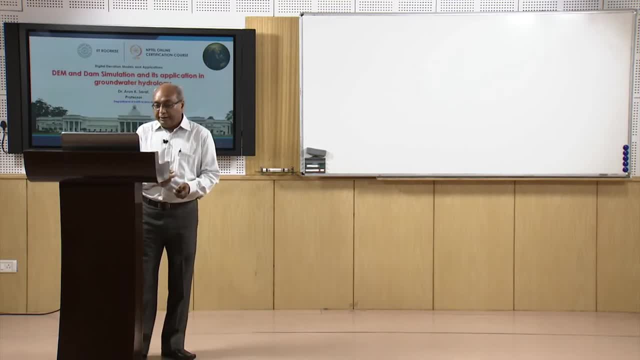 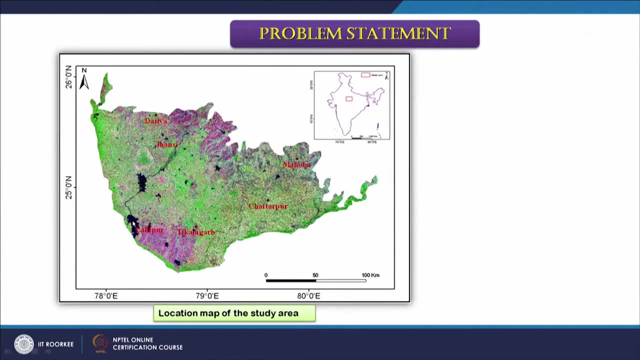 that benefit of digital elevation model derivative. This is the example in the same area as we have been discussing These two reservoirs, especially the Rajghat we have already discussed. So what we can do here is because this Bundelkhand. 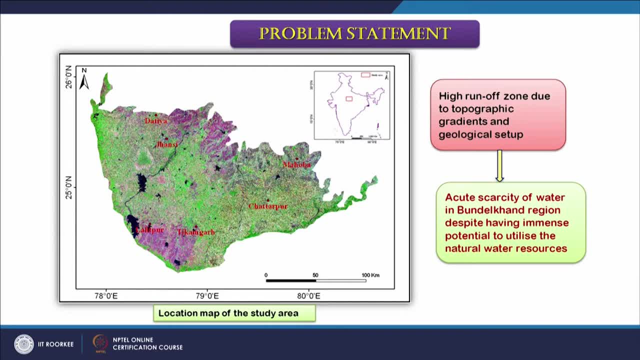 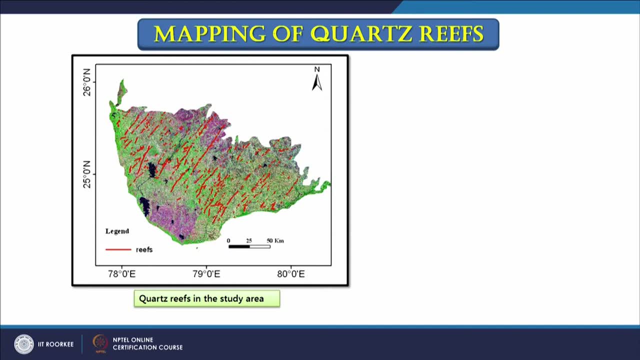 granite is having tens of or hundreds of these quartz reefs which are serving as a dam access, can serve as a dam access Already, serving for fuel And Damps Which are there in parts people have constructed, And these quartz reefs are running roughly East-West and so the Northeast, Southwest direction which have been delineated. 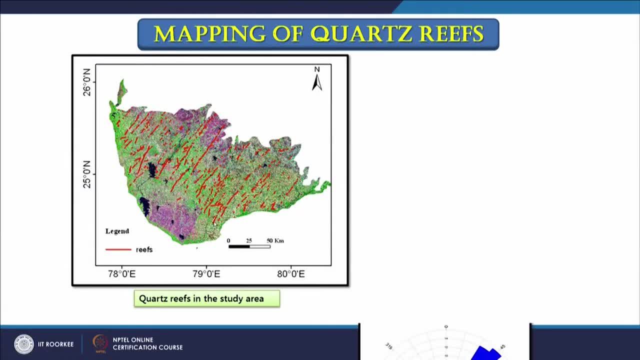 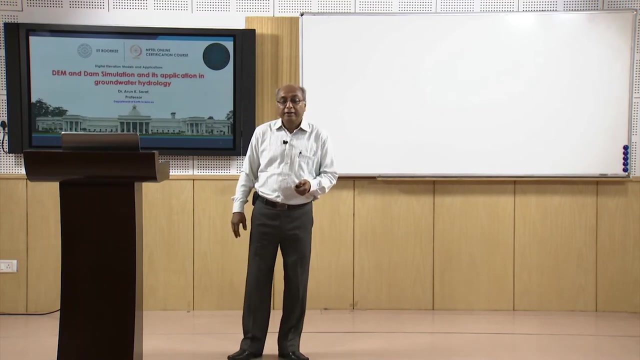 using satellite images as you can see these red lines and these can serve as these are the general directions of the quartz reefs and the major drainage which is going from from south east direction towards the north west direction. So this is, that means they are perpendicular to each other, and that can be exploited very easily. 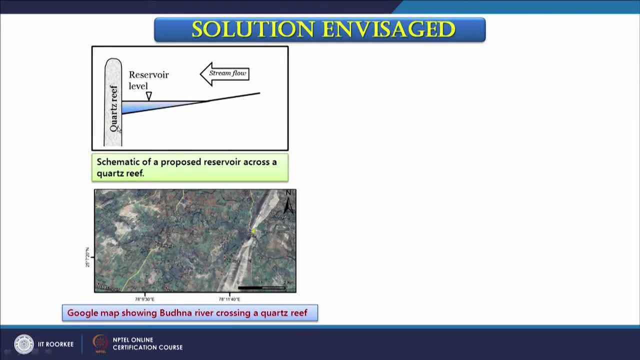 So this is the scenario here. through a schematic, suppose this quartz reef can serve as a dam axis if I fill with water. this is what the scenario I can have and as one quartz reef here in this example has been identified based on the Google satellite images study based. 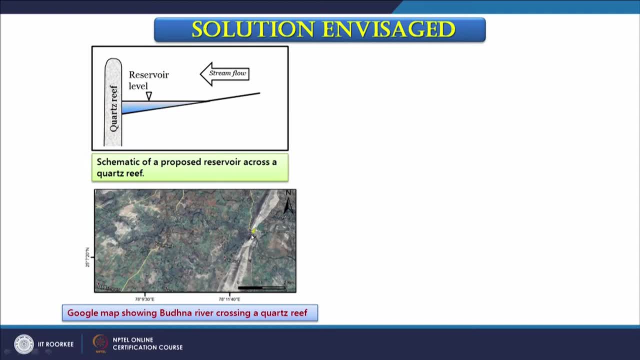 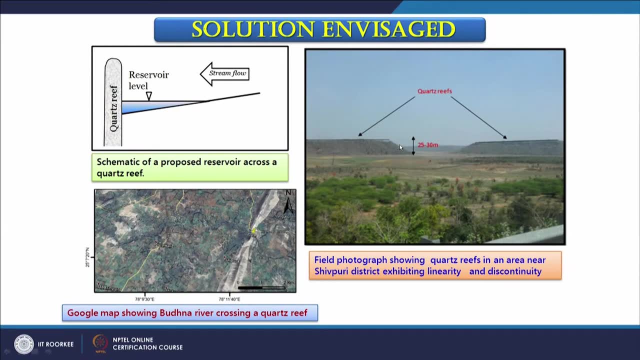 on that study we have identified there can be many such locations and we can simulated them. So this is the ground scenario. this is how this quartz reefs, which are about 25 to 30 meter height relative to that ground, and a stream is going across this. So if we plug, 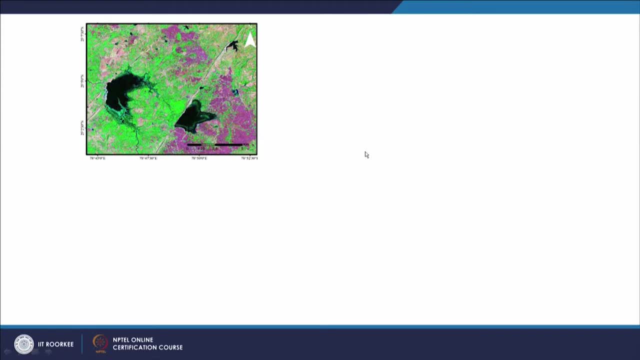 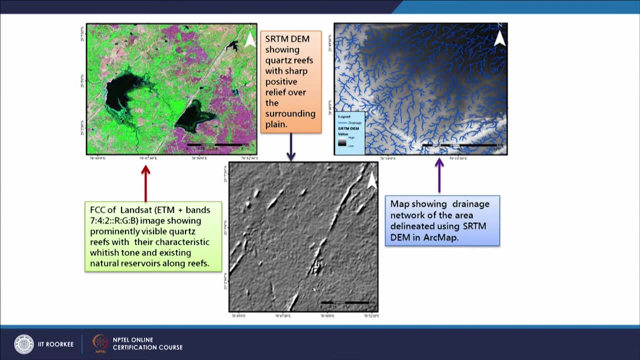 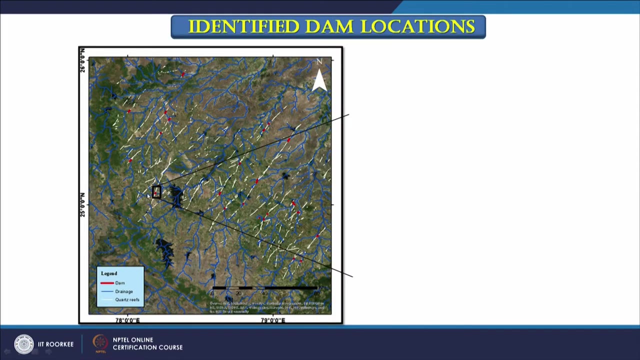 this one. Then in upstream we can have a reservoir, like these have been done in past and so we can. this is a shaded relief model of that part. drainage lines can be identified again can be derived from surface hydrologic modeling And we take example here and this is the scenario that quartz reef is running like this and 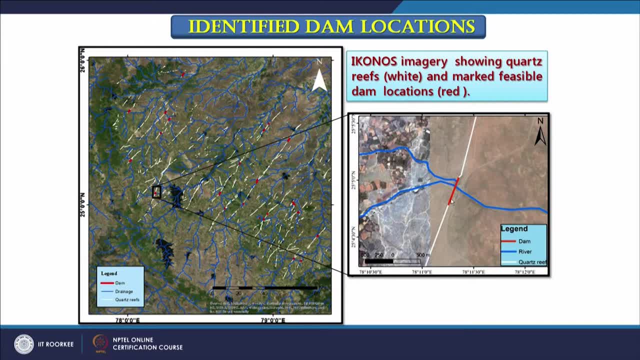 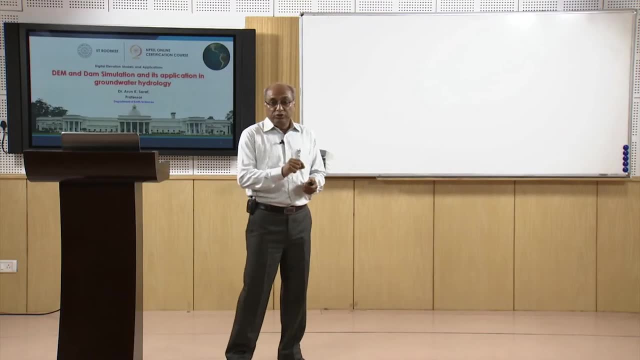 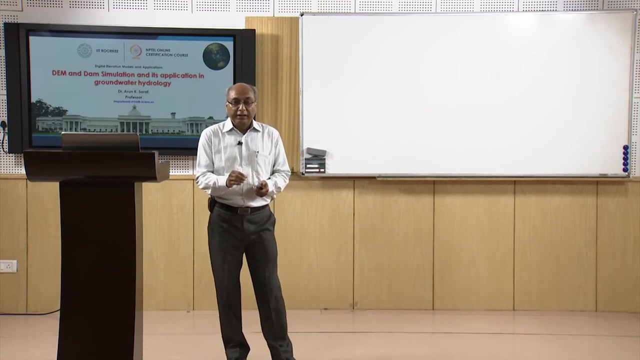 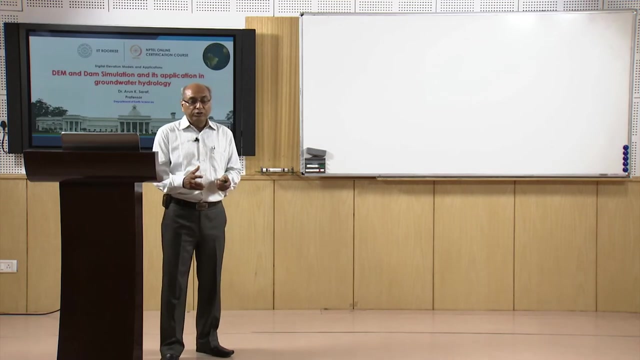 this is the dam axis, proposed dam axis for simulations, and we can simulate that how very much, where, how much area it will if we fix some height, and then this is the scenario. So this dam simulation which we have just discussed, using a digital elevation model on a GIS platform, can give us for locations of small reservoirs which can be used directly. 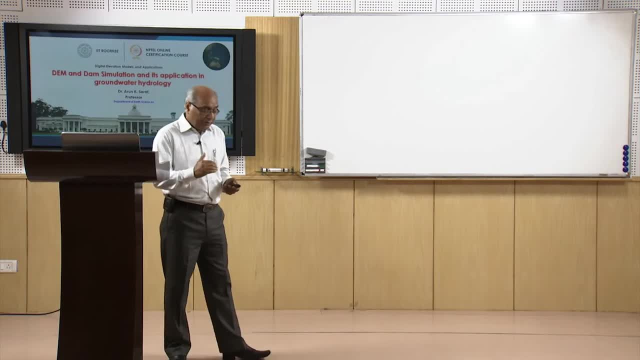 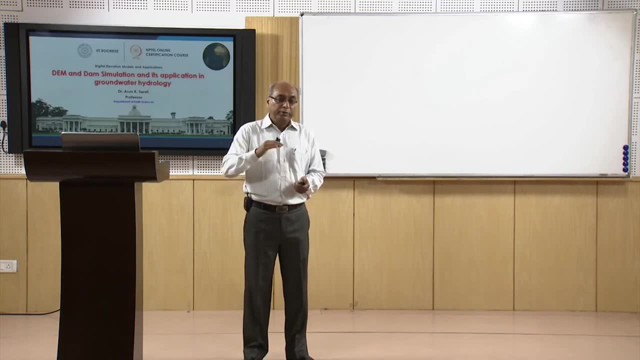 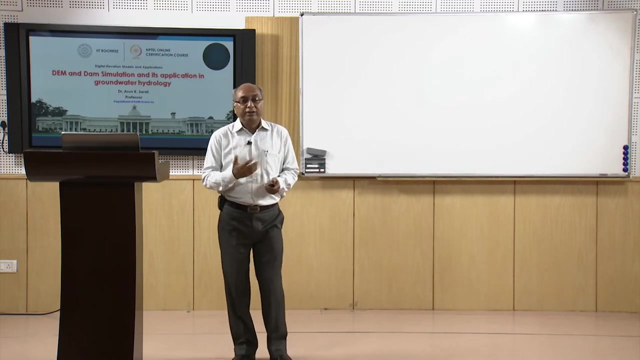 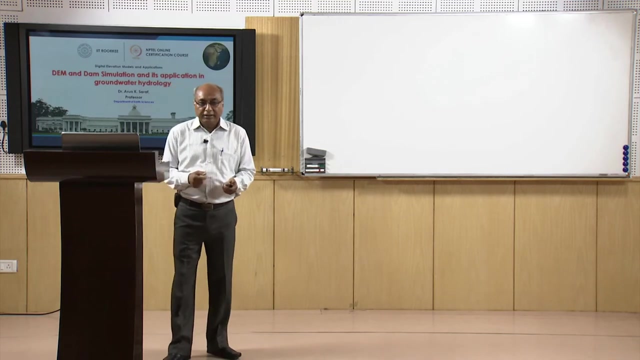 for groundwater recharge And the dam axis Is a Nature has already created in form of quartz reefs which are 20 or 30 meter height. So if we put this dam axis, plug that stream, along this dam axis or quartz reef, a reservoir can be constructed very quickly. also, one can see the cross section or profile along this. 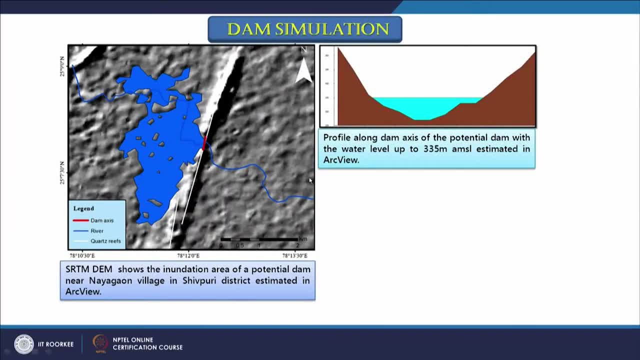 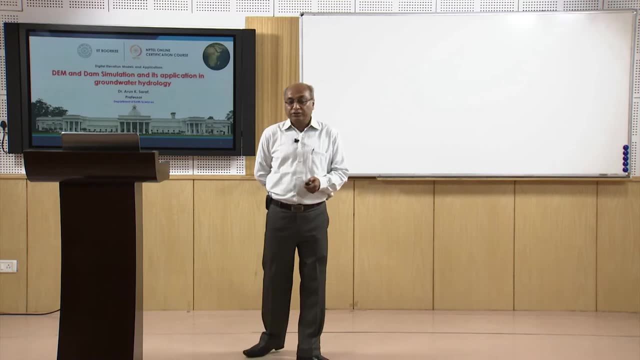 dam axis and still, if we want one, can increase the height. that means the inundated area of the dam will increase, the volume will increase. but whether that is required, whether that would be beneficial, all these things can be assessed before anything is really constructed on the ground. 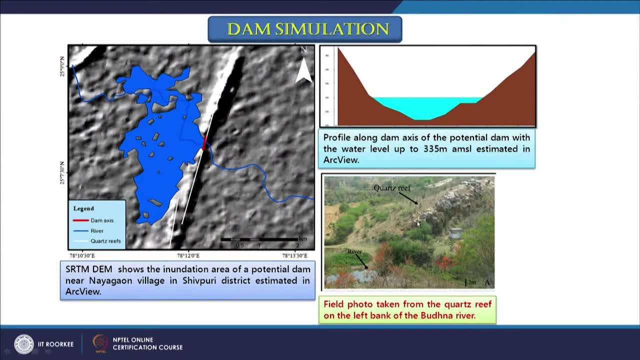 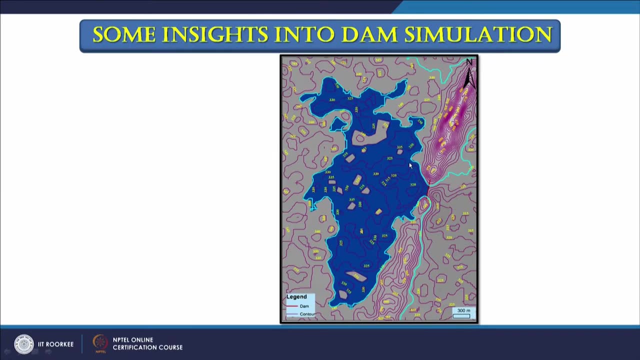 As a field photograph shows that this is the situation of the quartz reef and this is the water or river which is flowing or going across this stream. only thing it is required it has to be flood. only one bank is shown here. the other side is not in this photograph and also 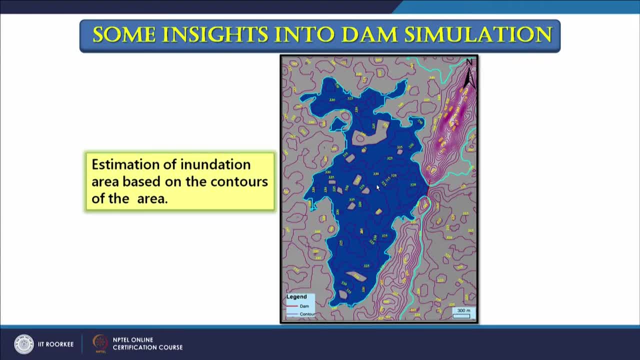 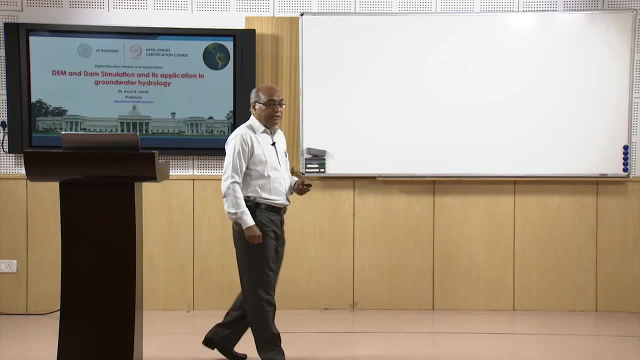 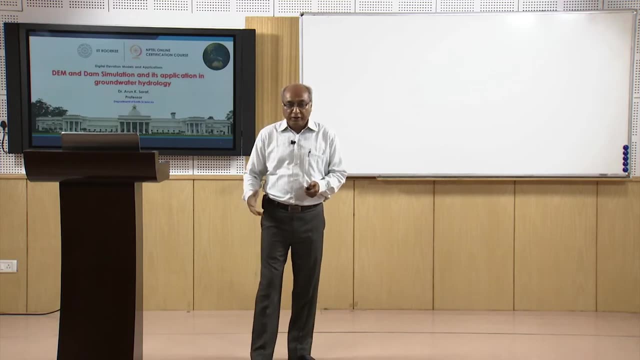 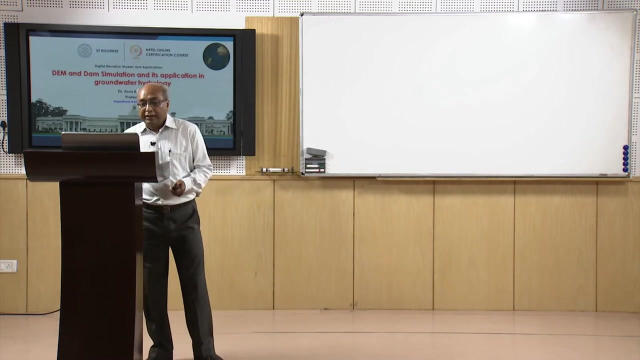 you can get about this estimation how inundations will occur at different water level in the reservoir. also employing the satellite images, one can estimate what is which are different land uses which will submerge if a reservoir is constructed here and if it can be shifted if it is required, then those things can also be done quite easily, as here. 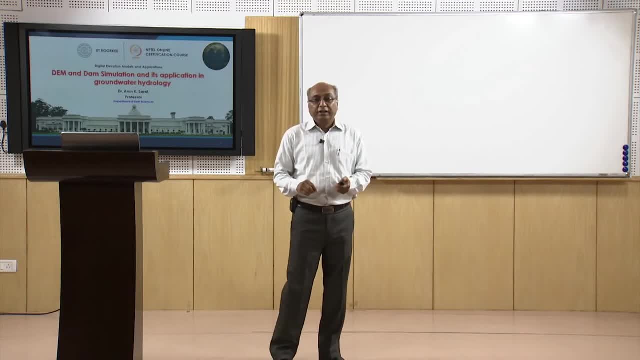 and shown in this particular Example. remember this thing: nothing has been constructed on the reservoir and this is the best example of modeling or simulation. what inputs we are having? a simple digital elevation model. in this case we may require relatively higher spatial resolution. digital elevation model may be 30 meter or 10 meter. digital elevation model and satellite images to estimate. 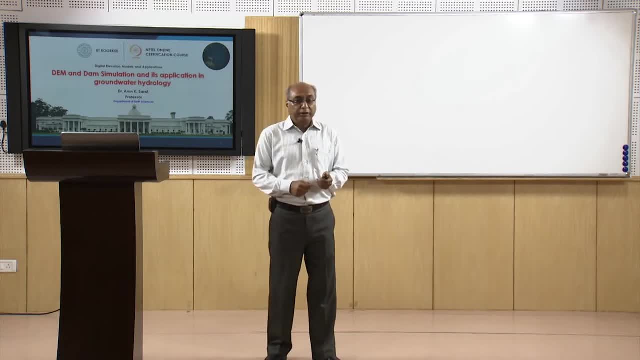 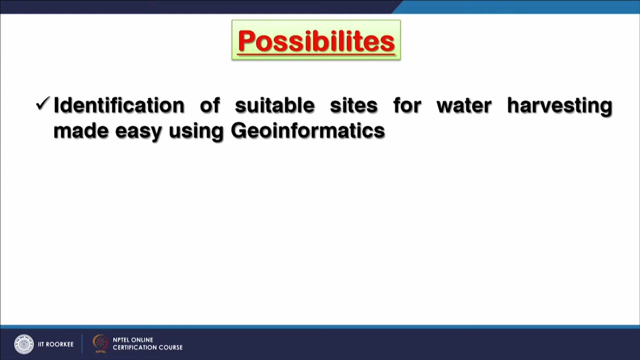 to predict many things which might happen In that particular area, especially focusing towards the groundwater recharge studies. So what are these? are the possibilities that we can identify suitable sites for water harvesting and using this digital elevation model and remote sensing inputs on a GIS platform. and 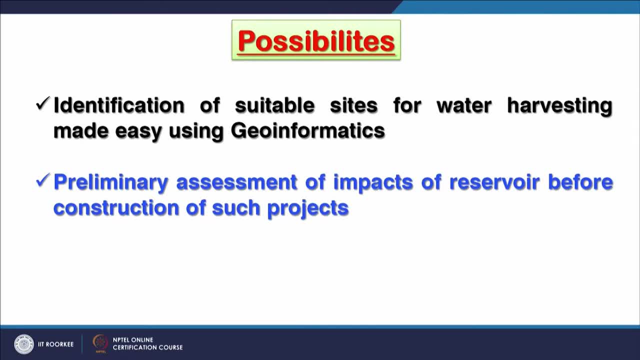 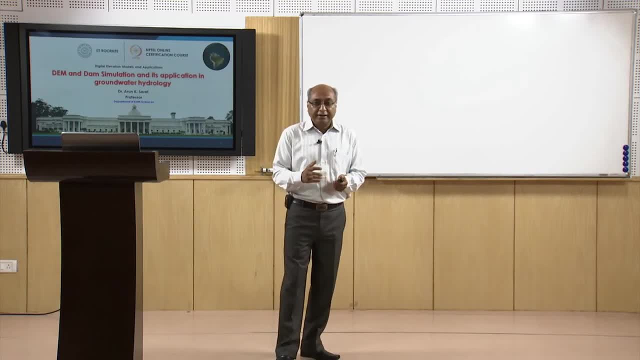 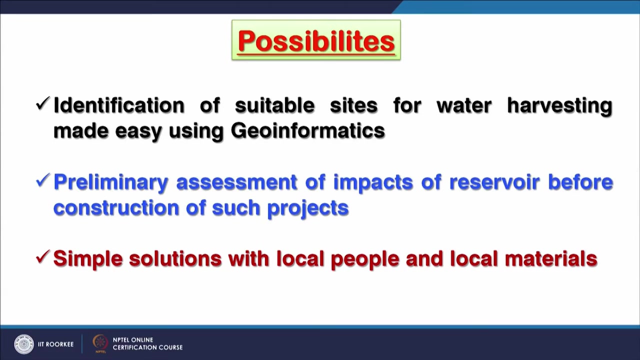 preliminary assessment of impact of reservoir before construction of such projects. So by looking the surroundings Satellite images we can predict that how much time it would take to take effects of these groundwater structures towards groundwater regimes through growth of vegetation. and simple solutions are possible as shown in or discuss in this lecture with the local people and 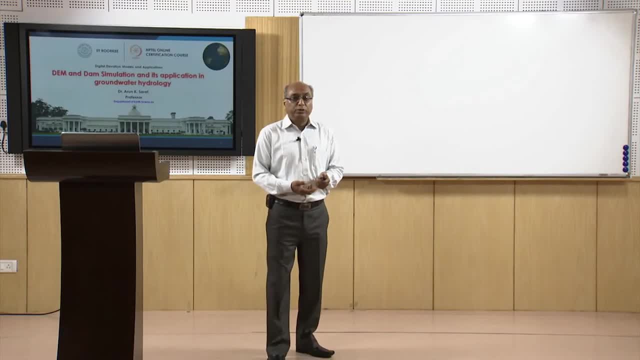 local materials which are available. nature has created few things like dam access in that particular part of the country. Only thing it is required: the identification of suitable sites, a simulation, and then the construction on the ground. One can use simply the Google map in which this terrain information in form of shader. 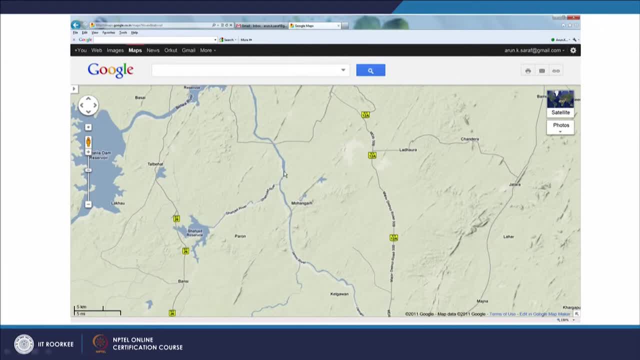 relief model is there also, the locations of streams are there and you know exactly where dam can like, for example here. Quad reef is running from northeast to southwest direction. this part is Going, this river is going unplugged, So if we can plug that one, a reservoir can be constructed very easily. 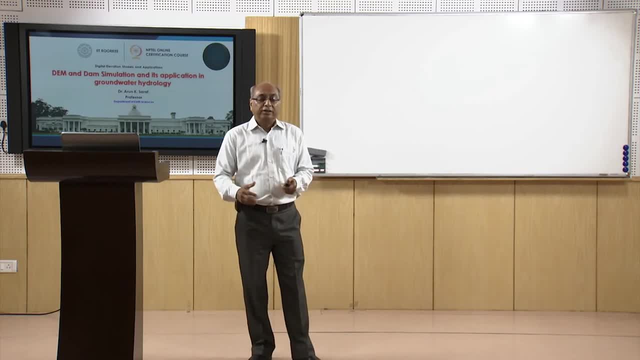 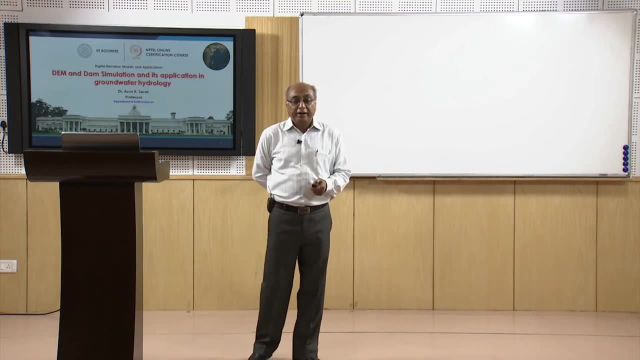 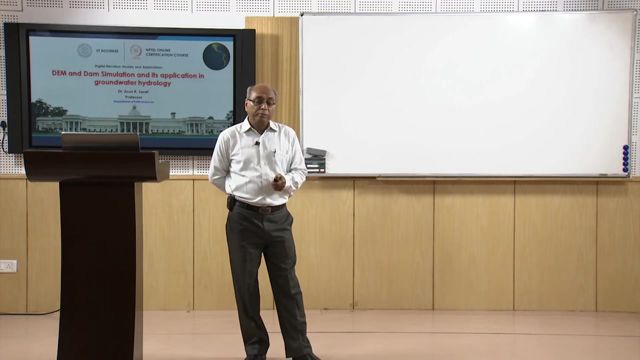 So the data is available, techniques are available. only thing is that it is required the things to be implemented on the ground and then we can augment the groundwater regime through these measures. though the rainfall- remember this we have a discussion about the rainfall- is quite sufficient. It is not too bad. 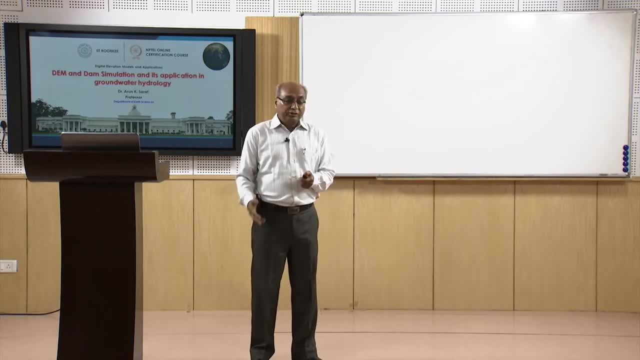 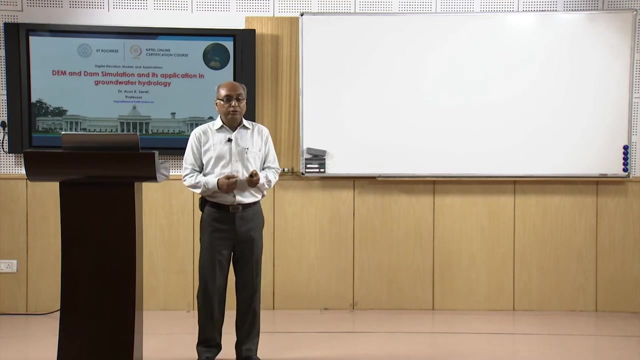 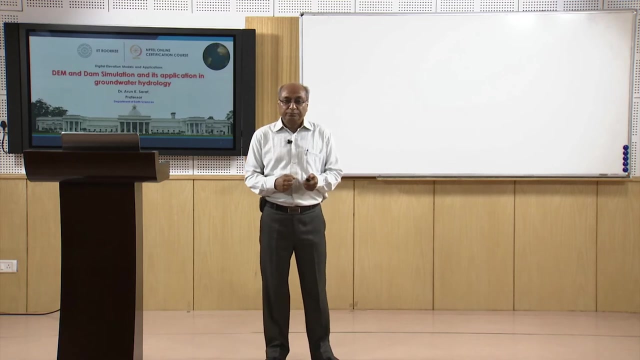 So rainfall is there, terrain is very suitable for such groundwater measures, only thing: it is required for the constructions and there are some other ways of employing, and very quickly. I would like to go again. this is based on digital elevation model, as we have seen that we can simulate or we can drive the drainage network. 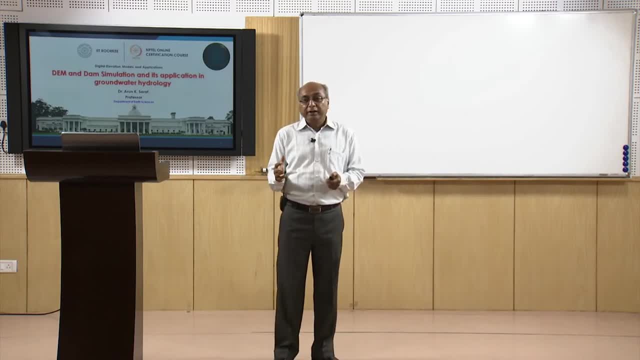 So what This is? what we have done is remember that we have discussed that in surface hydrologic modeling, one major assumption is that each drop of water has to flow on the surface, and so this is that means there is there are no losses, either to groundwater or to atmosphere. 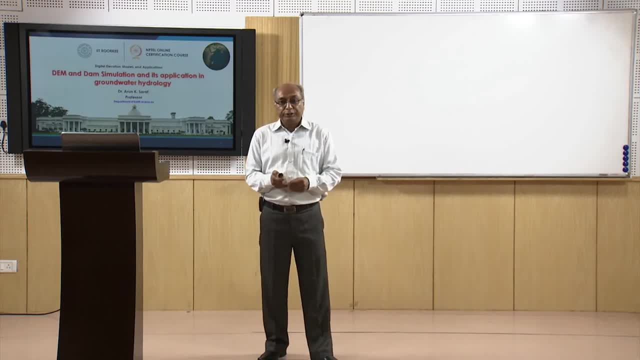 and that means there is no losses in form of evapotranspiration or neither infiltration or percolation, But this is the simulated drainage. that means the drainage network which we are driving based on surface hydrologic modeling using a digital elevation model in a GIS platform. 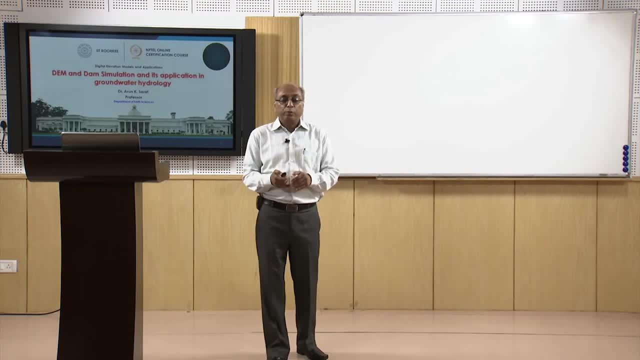 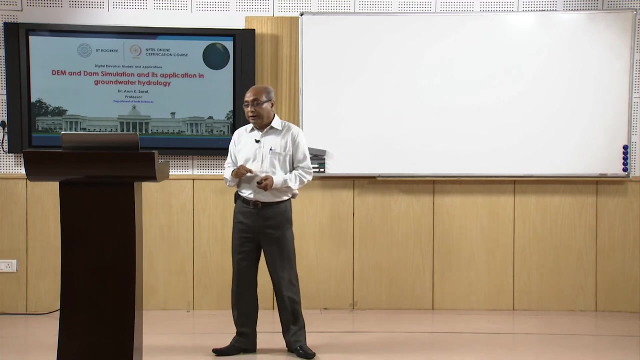 But natural drainage, which we can extract through topographic maps, will have some differences, because natural drainage is the real location of drainage present on the surface, whereas the simulated drainage will have some mismatches and this mismatch we have exploited. So this surface hydrologic modeling based on DEM and the drainage network coming from 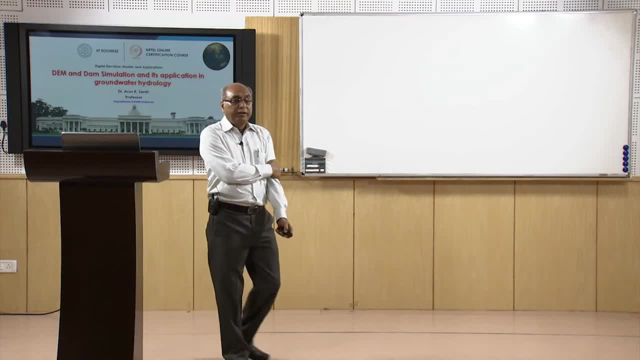 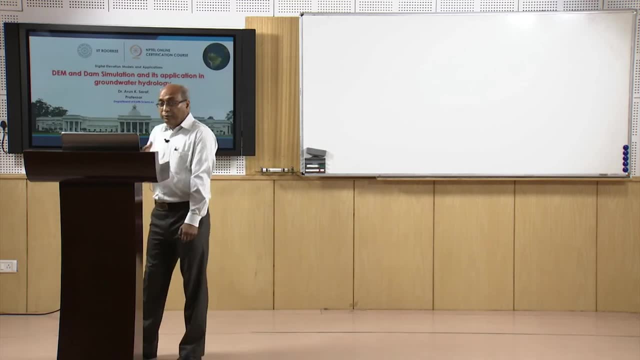 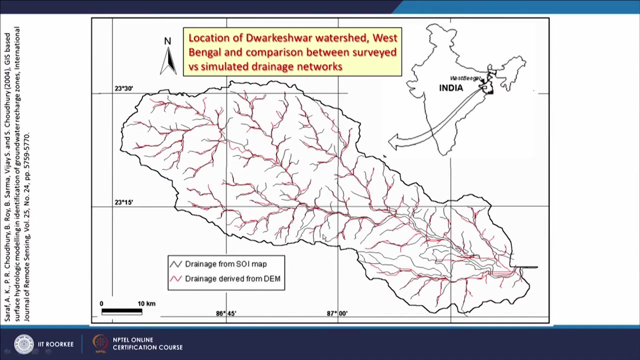 drainage from topographic maps have been exploited again, targeting the groundwater towards groundwater studies to locate which are the areas in a particular watershed are suitable for groundwater recharge. One example from West Bengal of Bankura district. What we see here in the background is the black colour drainage network which you are. 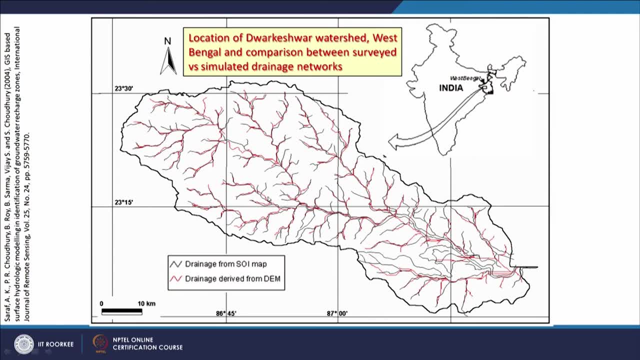 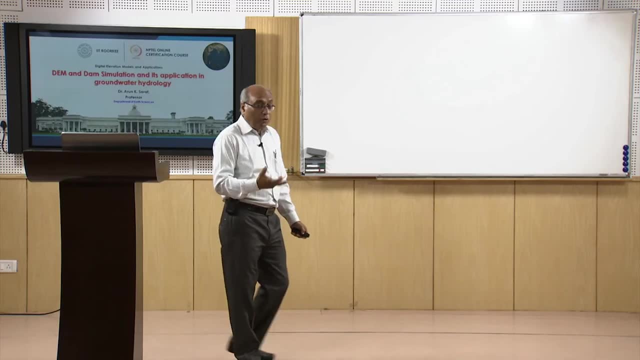 seeing is the drainage which has been digitized using survey of India toposheets of 50000 scale and over which the red colour one which you are seeing is the simulated drainage based on surface hydrologic modeling, Because the assumption there is the water has to flow on the surface. 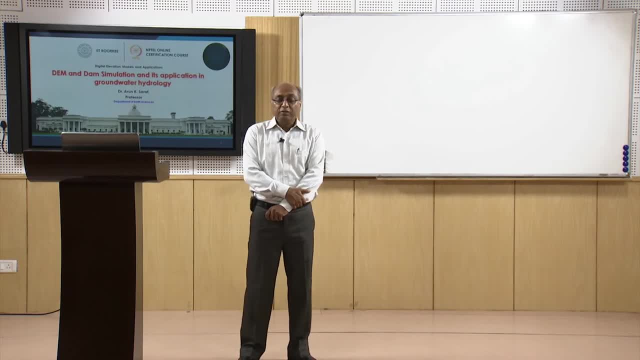 But in natural drainage that assumption is not there and therefore there is likelihood that there might be. if we assume that loss to atmosphere remain in a small watershed, remain uniform, then whatever the losses which are occurring are due to towards, for because of groundwater recharge, And therefore there should be some mismatches, and this is what we have observed in this. 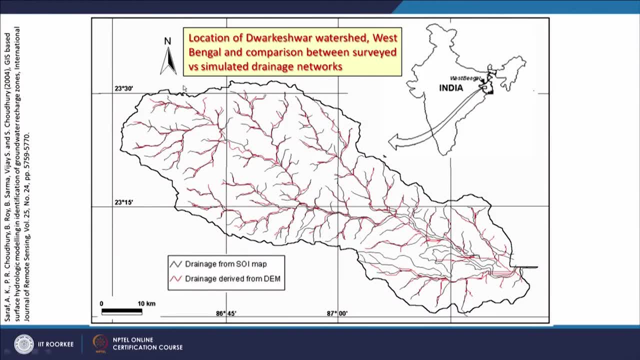 particular example that in the upstream part- this is all hard rock terrain- the natural drainage is following what the model drainage is, or simulated drainage. That means there is no loss of water towards the groundwater regime, whereas in the downstream area there are large mismatches and that means the water is not following the natural drainage. 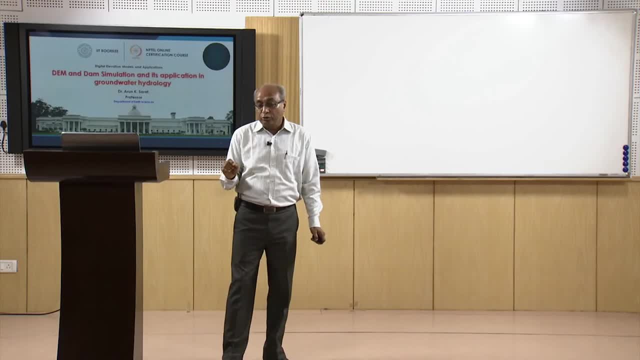 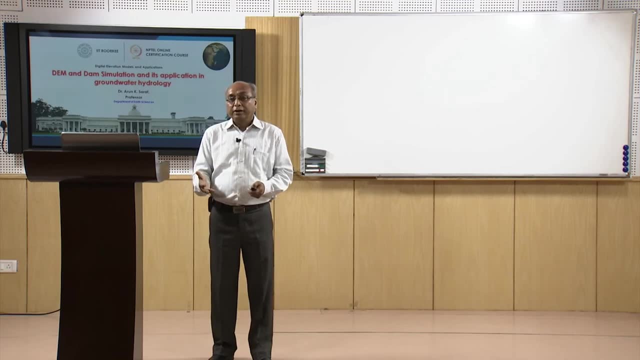 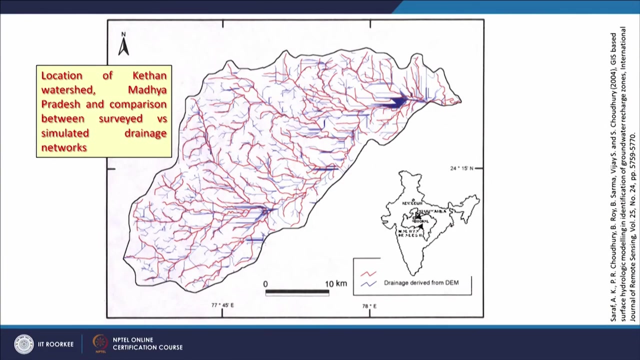 is not following the model one and that means there is a loss to the groundwater And in fact this loss we can picked up for the sites suitable for For groundwater recharge locations. so these are the sites which may be another example here, when we overlay these two, this simulated drainage and natural drainage, the mismatches. 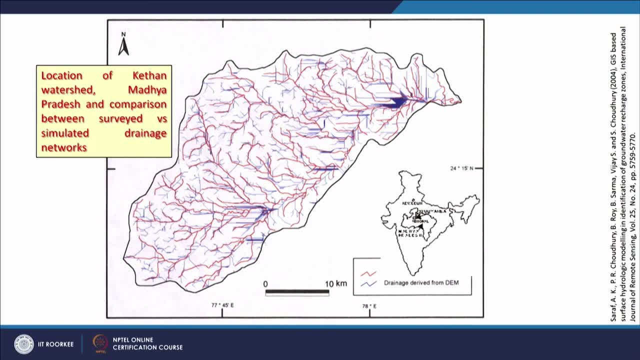 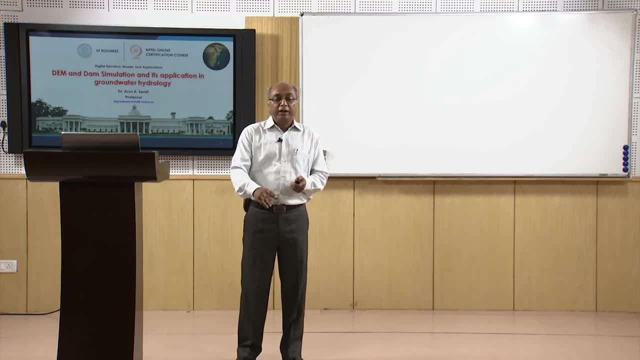 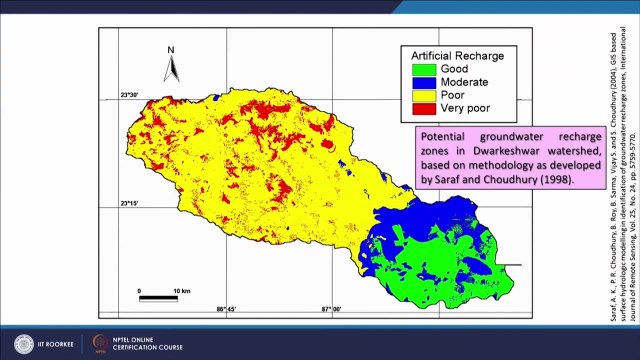 can be identified very easily And wherever the mismatches, that means blessing in disguise. where are the mismatches? we can exploit those mismatches and find and these are the probably the suitable sites for groundwater recharge, And this is independent. This was created without involving the drainage and this is what was seen that in this part. 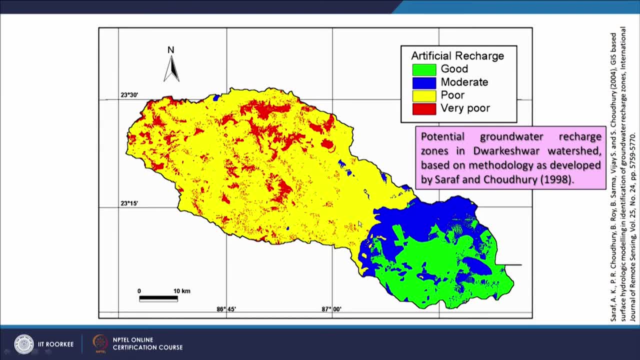 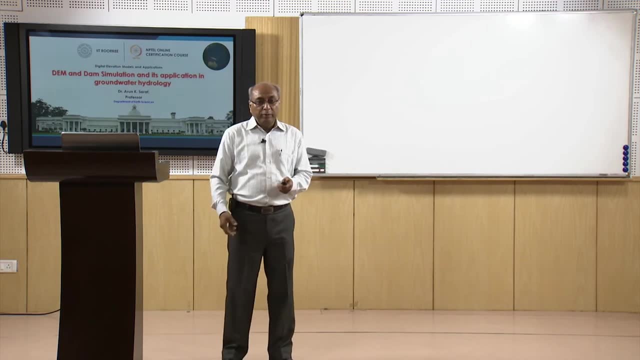 these are not suitable for any groundwater recharge structures, whereas this blue or green parts are most suitable where we have observed that the drainage and simulated drainage and your natural drainage had the maximum mismatch. So, likewise, employing a surface hydrologic modeling and a DEM, We can get such a analysis very quickly. 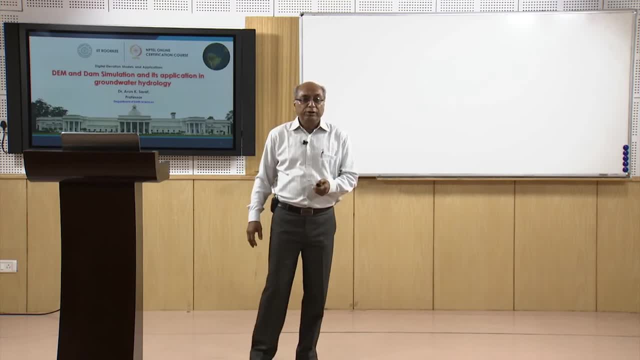 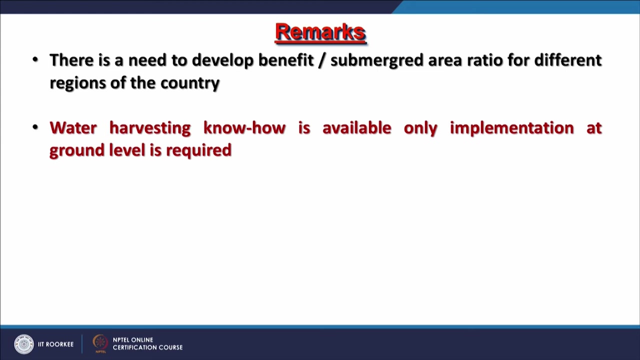 So there is a overall, there is a need to develop a benefit, some much ratio, that index for different parts of different regions of the country, So we know exactly how much land I have to invest for such structures, how, what benefit I will get in the downstream or the vicinity of a reservoir, future reservoir and water. 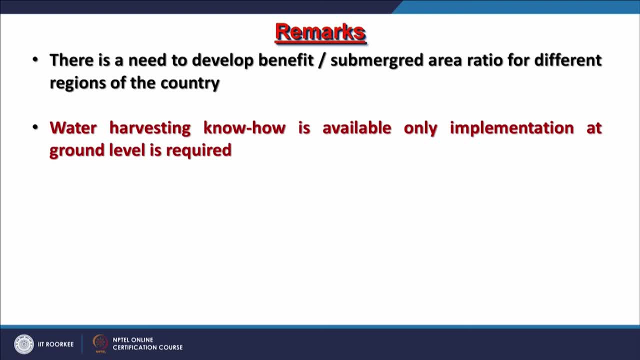 harvesting And know how is available that we know. the only thing: it has to be implemented on the ground. We can identify suitable sites for water harvesting or groundwater recharge, and the preliminary assessment of reservoirs can be done through on GIS platform using the surface hydrologic. 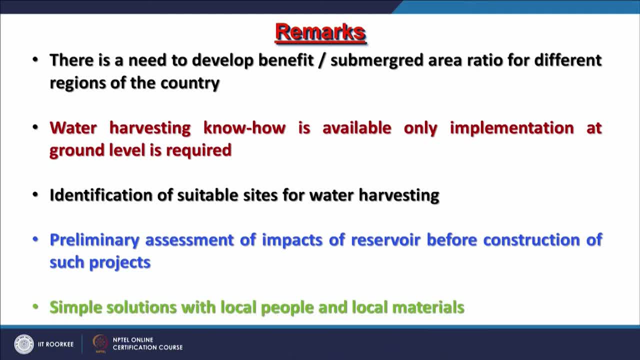 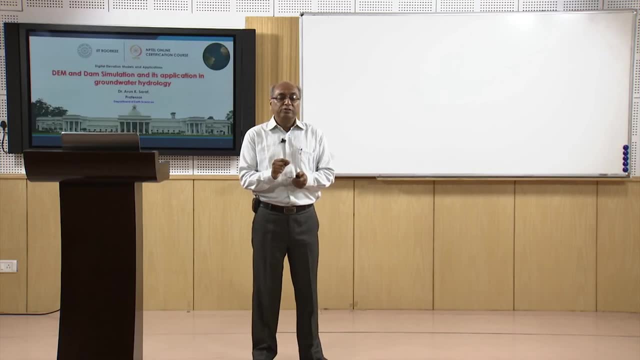 modeling and your digital elevation models and satellite images. And this is the repeat, The simulation, The simple solutions with local people and local materials. that means we started with. if we increase 1% of groundwater storage, we can solve the problem of groundwater in this.